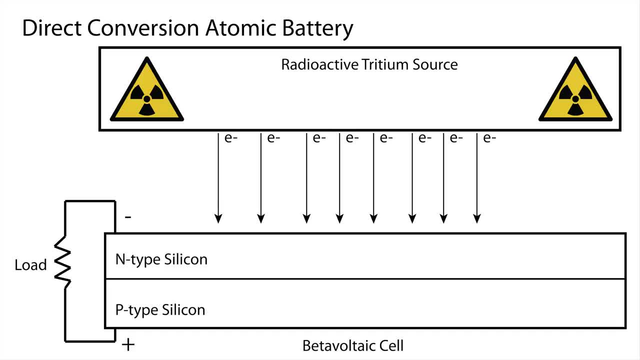 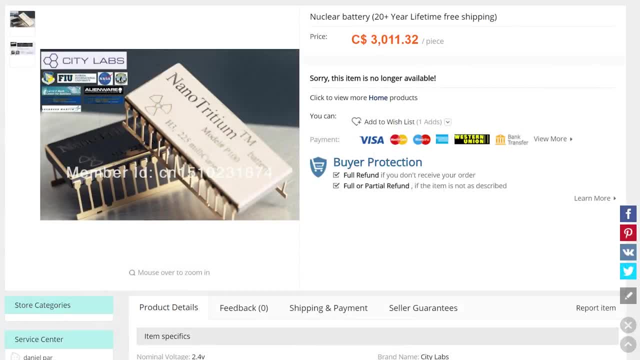 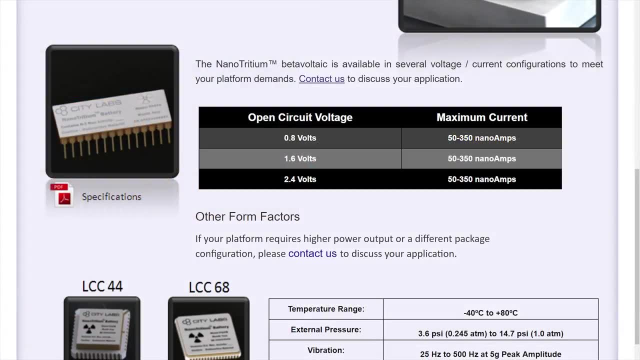 But instead of photons it absorbs beta particles. It is thus called a beta voltaic cell rather than a photovoltaic cell. My inquiries into the exact pricing were ignored, but you can find them online from resellers for $3,000.. In terms of power, their website lists their top unit as a voltage of 2.4 volts with a short circuit current of 350 nanoamps. 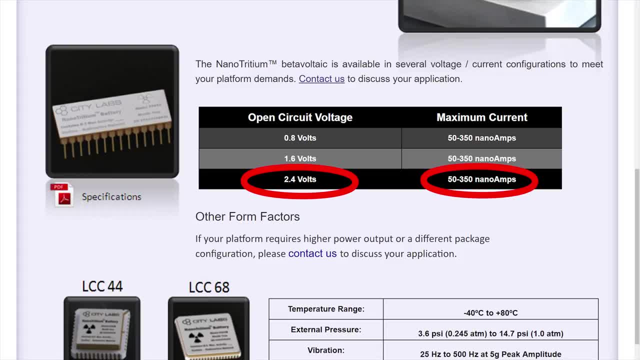 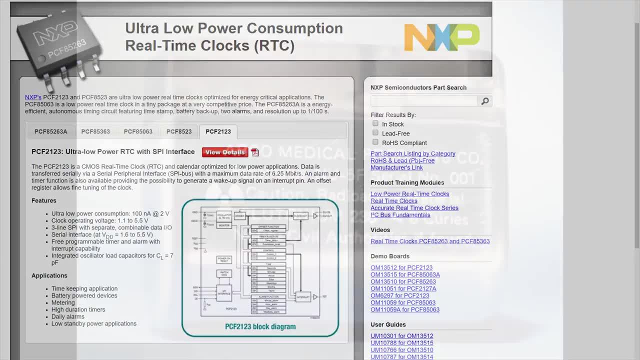 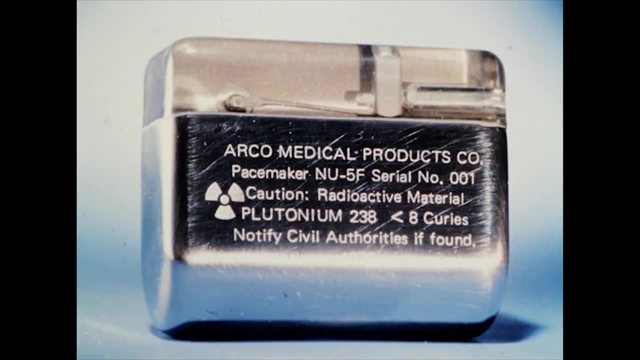 This is quite small, but it's meant more for lower power devices like the memory or clock circuits in highly critical machines where chemical batteries are not as reliable. Other uses include medical implants like pacemakers or remote sensors, where changing the battery is not physically allowed or even possible. 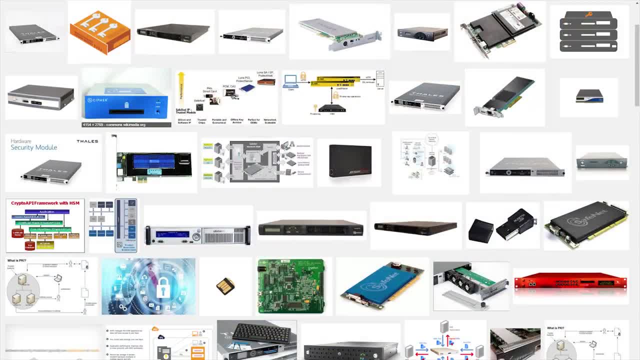 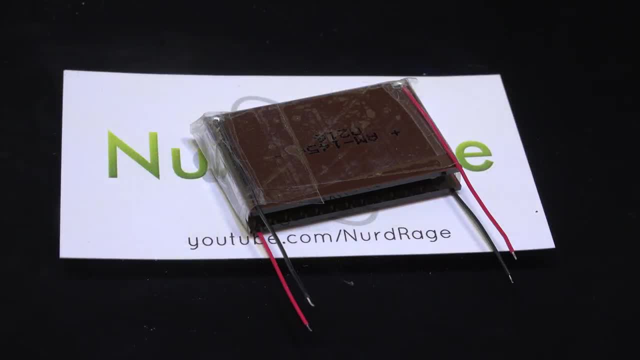 In hardware security modules. changing the battery isn't allowed for security reasons, so the battery must last on its own for the lifetime of the device. Let's try and make our own nuclear battery and see how it compares. Let's try and make our own nuclear battery and see how it compares. 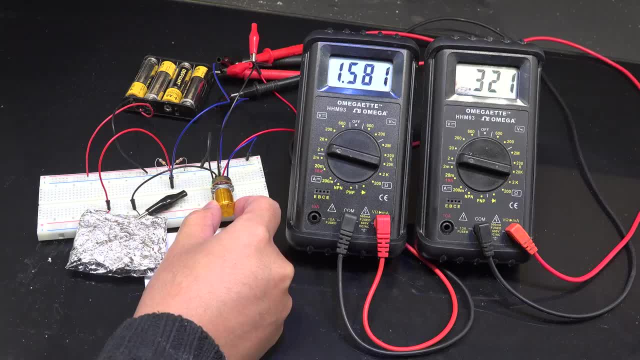 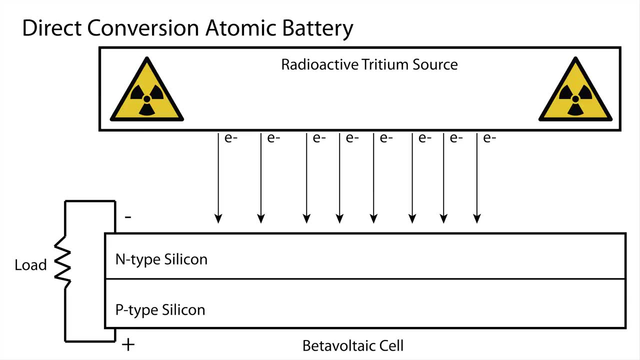 Let's try and make our own nuclear battery and see how it compares. It'll likely be more expensive and less powerful than the device from City Labs, but we're here to explore the science Now. the City Labs device is categorized as a direct conversion radioisotopic battery in that the radiation directly interacts with the beta voltaic cell to produce power. 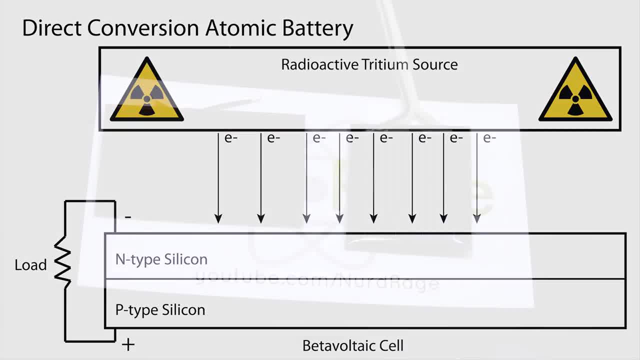 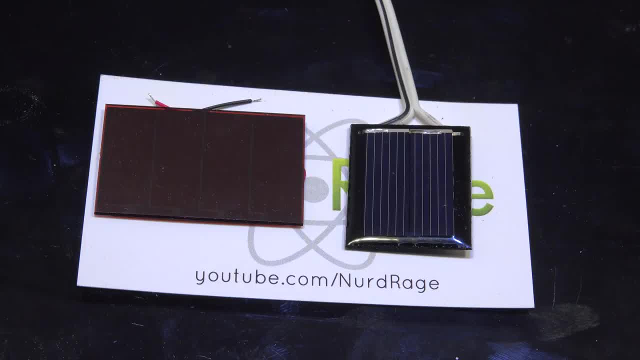 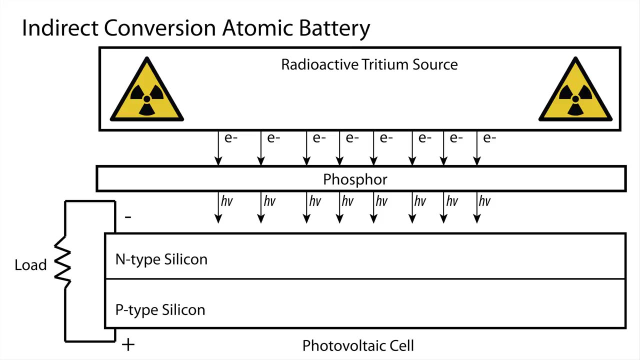 There isn't a commercial source of beta voltaic cells, so we're going to have to use a photovoltaic cell. But photovoltaic cells only convert light into electricity, not beta radiation. We need to convert beta radiation into light first. This technique is already well known and is categorized as indirect conversion. 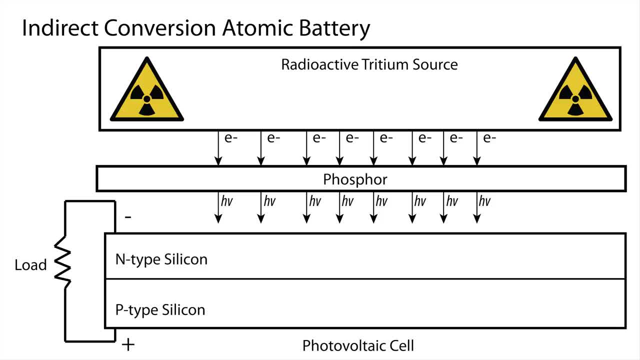 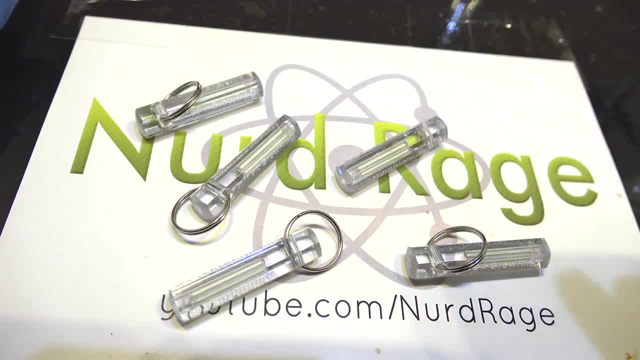 The simplest way of doing this is to put a phosphor in front of the radiation source which converts it to light. Fortunately for us, there is an easy to get commercially available supply of safe radiation sources that have light conversion already built in. It's these tritium keyring lights. 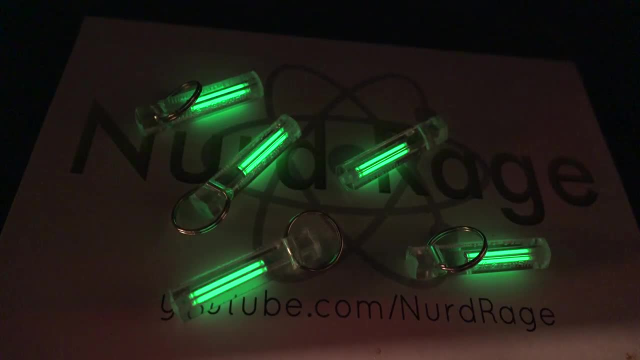 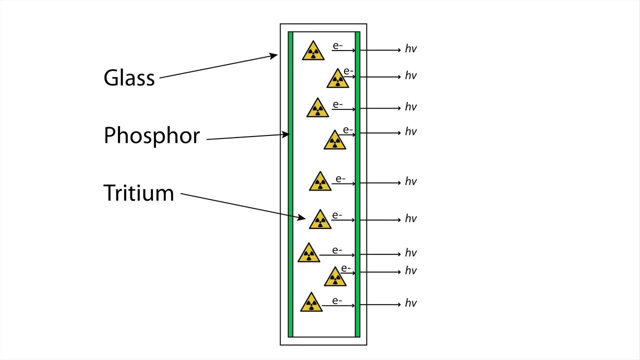 You can also find them as fishing lures, gun sights, emergency signs, military lights and so on. They work by having a sealed glass vial of tritium gas and internal phosphor coating. The radioactive tritium gas emits beta radiation that strikes the phosphor and emits light. 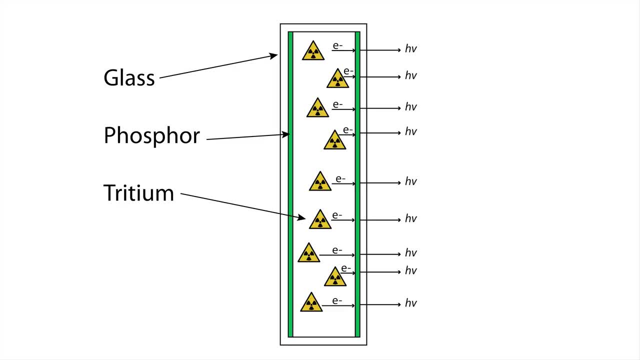 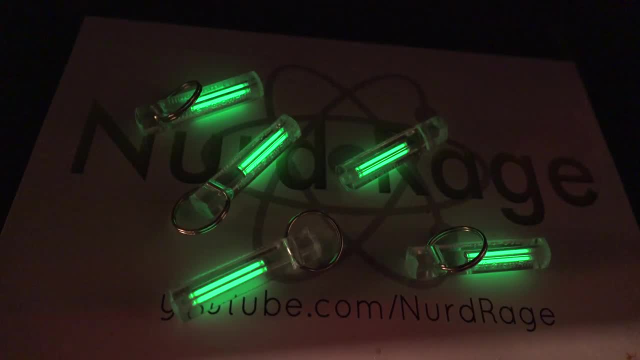 So the hard part of generating light from a radioisotope has been solved for us. This lets us avoid the safety issue of handling a radioactive gas. Now i bought mine online and they come encased in plastic. The actual tritium vial is much smaller. 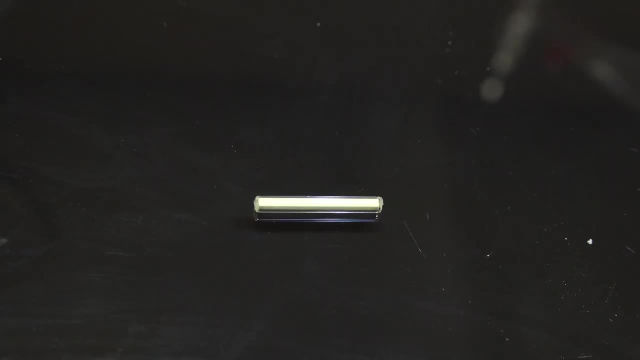 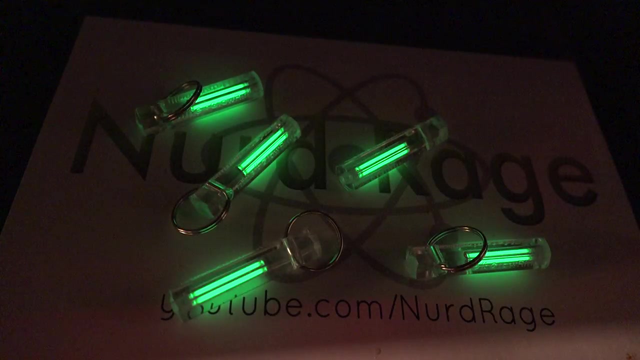 I could have bought the vials directly. The seller i got these lights from must have had a pricing error because they were selling for less than the price of the bare vials. So i took advantage and bought fourteen before they pulled their listing. Presumably they realized our mistake. 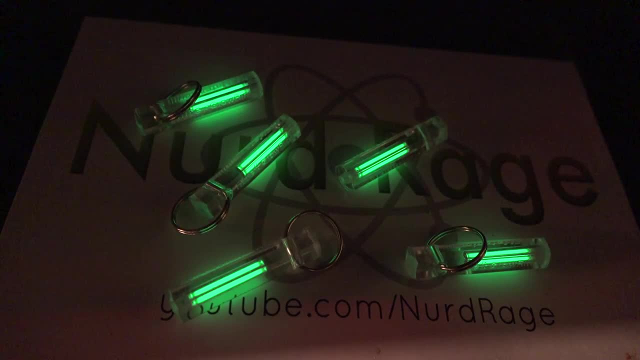 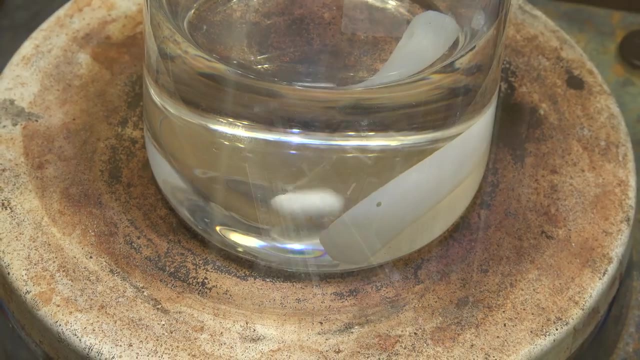 Yeah well, score one for me, But i still have to remove the plastic casing to get the vials. Now the casings dissolve into chloromethane solvent, but only sparingly. To help along the process i use the soxhlet extractor i've shown in a previous video. 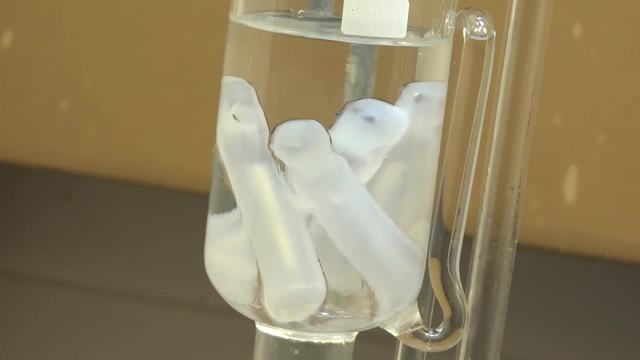 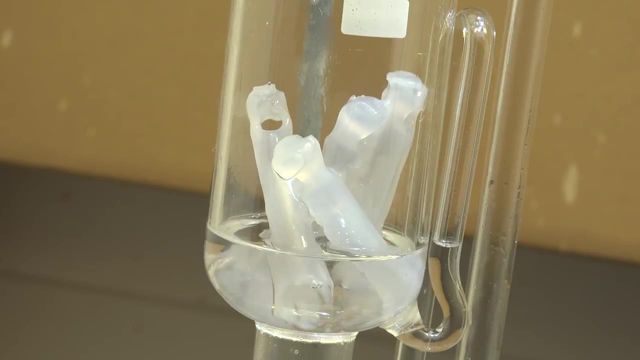 Briefly, the extractor constantly exposes the tritium lights to freshly distilled dechloromethane and then drains it away, where it is reboiled and dissolved again. Thus i can use very little dechloromethane but thoroughly dissolve the plastic from the lights. 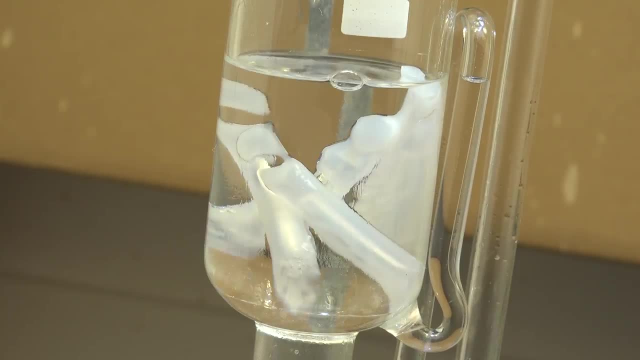 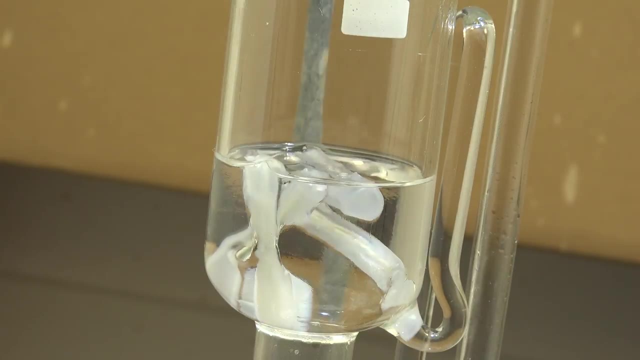 Another reason why i use the extractor rather than just stirring with lots of dechloromethane is that the extractor is very gentle. There isn't a fast spinning stir bar to smash the delicate glass vials of tritium once they are exposed. 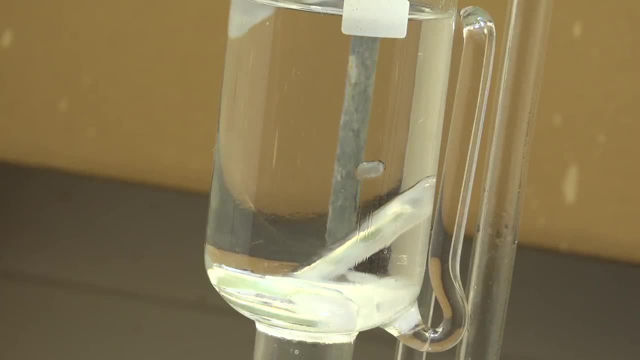 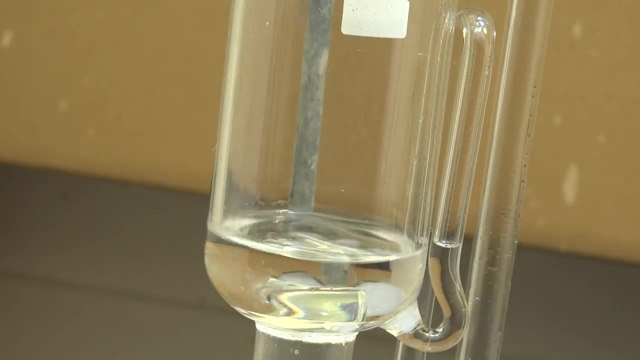 While the radioactivity is small, it's not a good idea to take any chances Now. i can do tritium vial decapsulation cheaply because i already have a soxhlet extractor. If you're making your own nuclear battery, then just buy the vials directly. 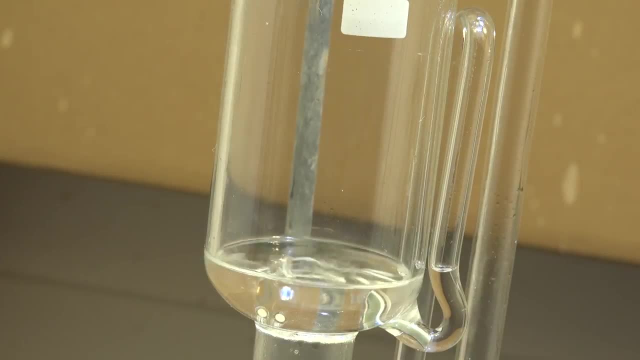 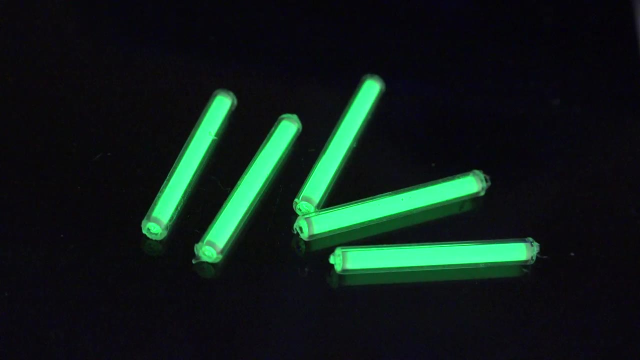 Unless you take advantage of pricing errors like i did, the naked vials are usually cheaper than the encased lights. Anyway, there we go, tritium vials. Before you get too excited, they're not actually as bright as my camera suggests. 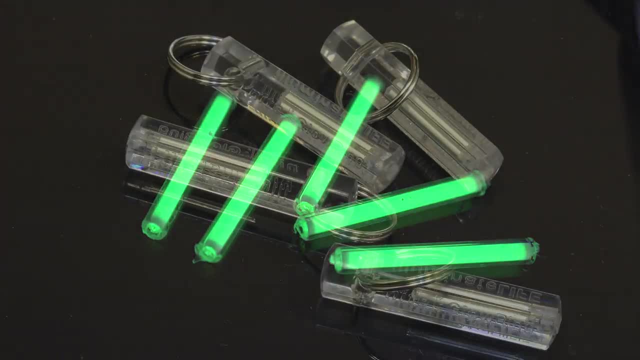 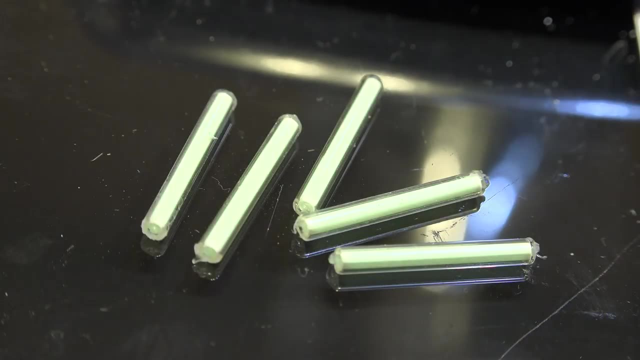 I'm just maxing out the exposure settings. Anyway, i have more to go, so i'm going to put in a fresh batch and keep going. Now i noticed my vials had some insoluble rubber at the ends. Presumably it's silicone rubber and likely used to protect the vials from damage by cushioning from hitting the ends. 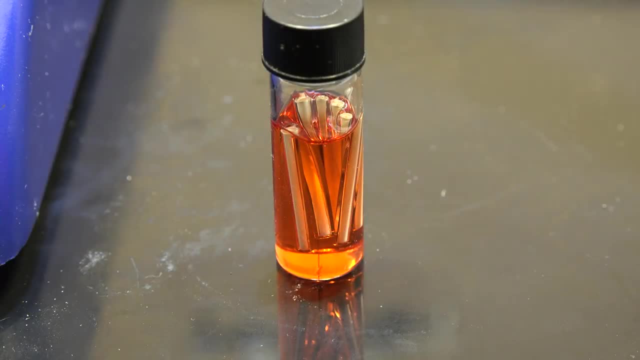 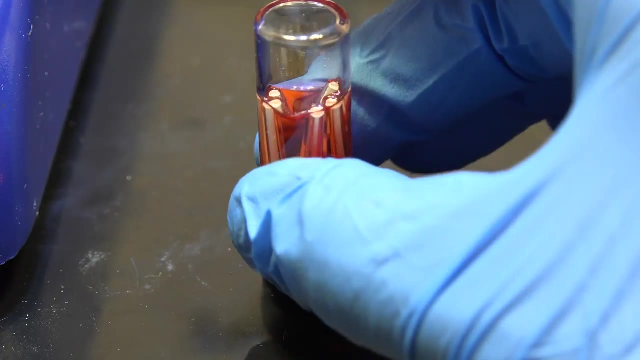 If you want, you can remove them by placing the vials in concentrated sulfuric acid. Silicone rubber is easily destroyed in sulfuric acid and after an hour they can be removed and washed with water. Nonetheless, this is strictly optional and not actually necessary. Now we have cleaned tritium vials. 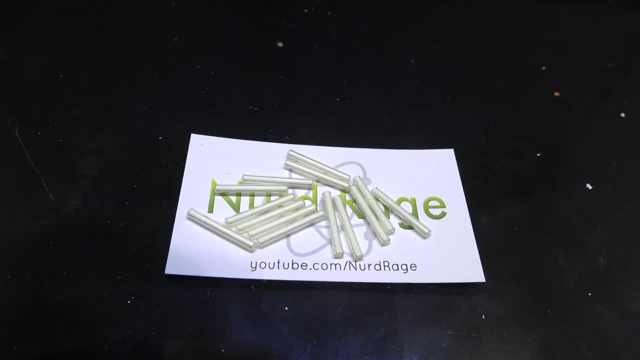 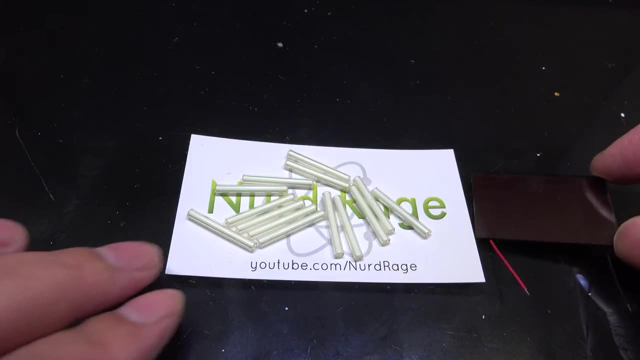 And here we have it: Fourteen vials of tritium. Turn off the lights and make sure they work and haven't leaked. Now, to generate our power, we put them in a solar cell. I'm going to use this amorphous silicon type solar panel you might find on calculators and other devices meant for indoors. 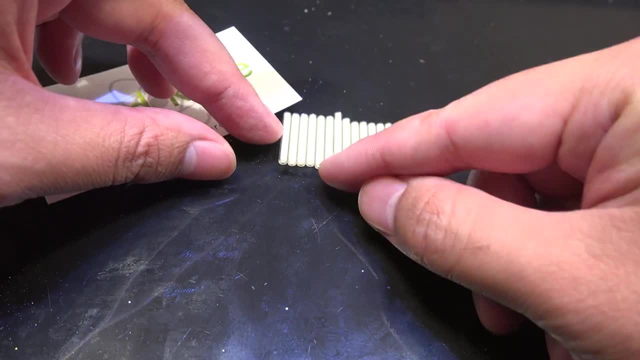 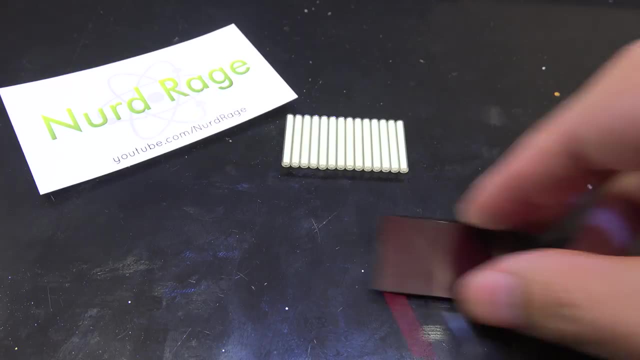 Don't worry, i'll test the more efficient mononucrystalline solar panels later. Now i intend to build a box, but for now a quick and easy way of mounting the tritium is to first align them so they match the shape of the panel. 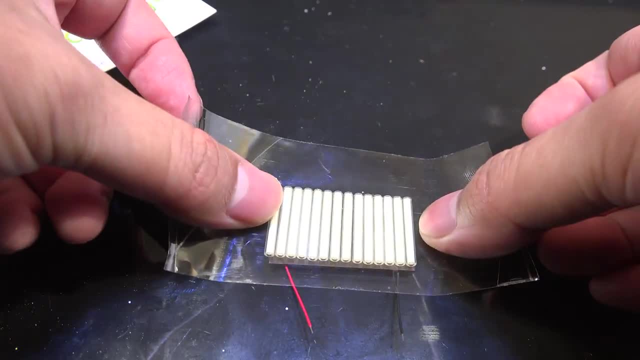 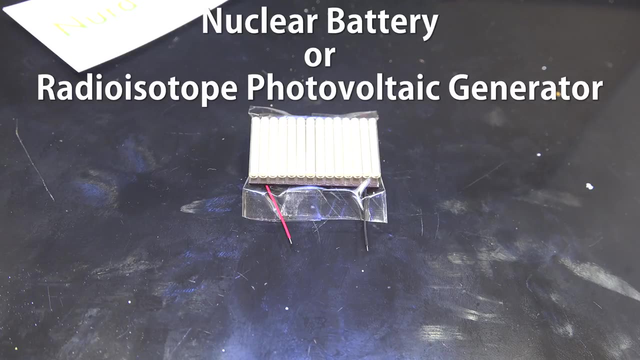 And then taking some tape and picking them up, Make sure they match. Now just place the panel on them and tape over, And now we have our simple nuclear battery. This is also called a radioisotope photovoltaic generator. It's not a thermoelectric generator, because it doesn't use heat, but just light. 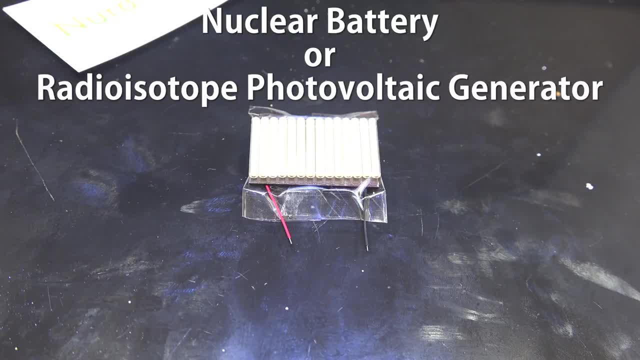 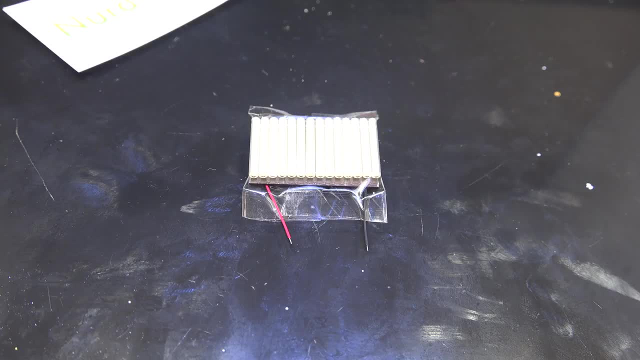 And we're using a photovoltaic cell and not a thermoelectric one, So it's photovoltaic. Now i'm going to put a second panel on top in the final version, but for now this is good enough for performance testing. To ensure we get accurate results, we encase the unit in aluminum foil to prevent it from leaking. 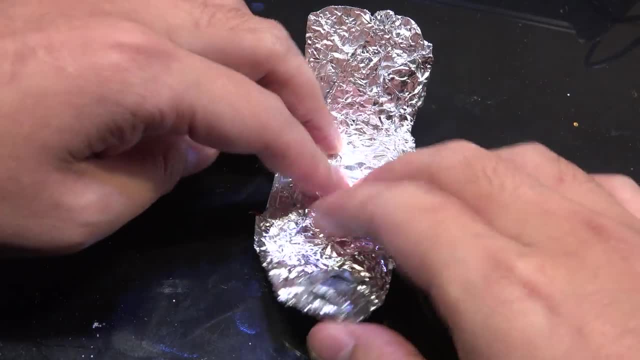 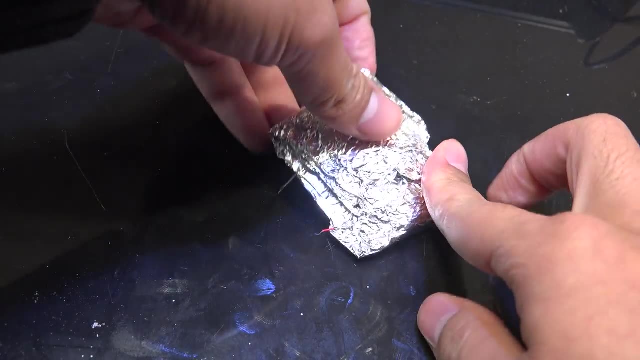 And we're going to block outside light. Make sure the lead wires stick out Now. outside light can only help us in terms of total power generation, but we want to focus on just the nuclear energy part for our analysis. So let's get some performance numbers. 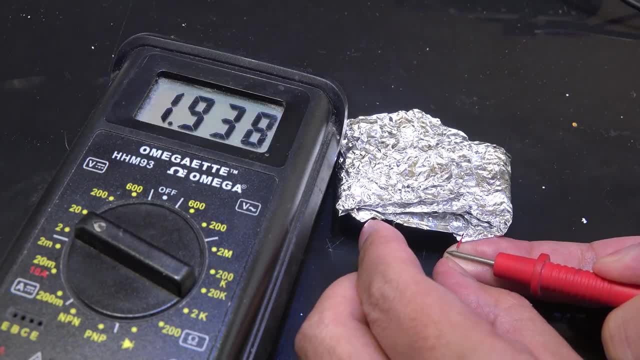 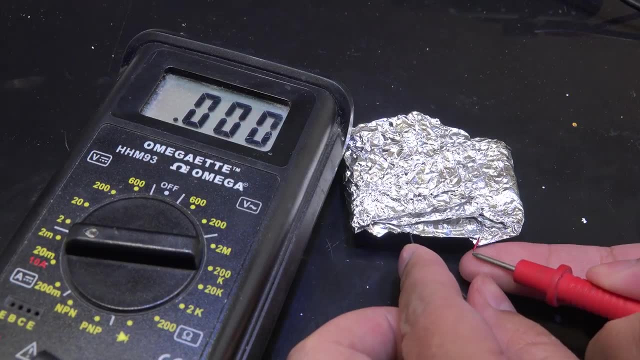 We can measure the voltage and the panel seems to be generating around 1.9 volts, So we're off to a good start. Let me switch over to measure current. Let's see what we get, And it looks like we have extremely low current. 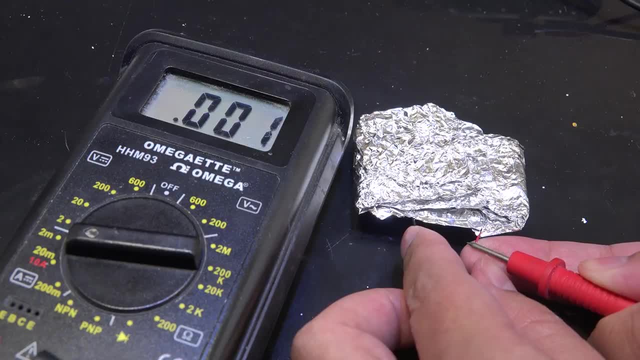 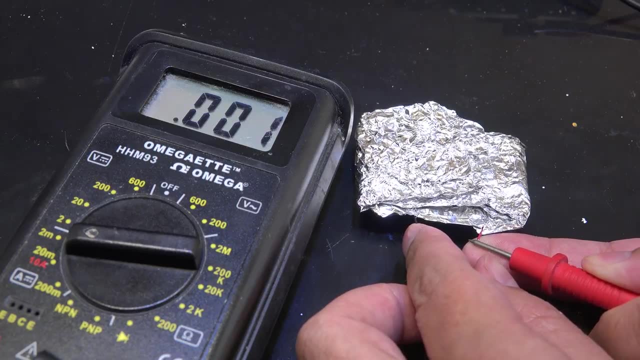 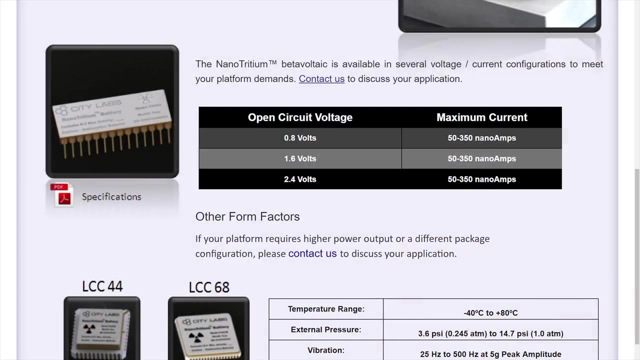 Only 1 microamp. Now this reading is likely completely inaccurate. For all we know, our device is generating half that current and my meter is rounding up. My meter could even have measurement errors and the true value could even be lower. Before you get too disappointed, keep in mind: the professional device built by city labs only produces 350 nanoamps. 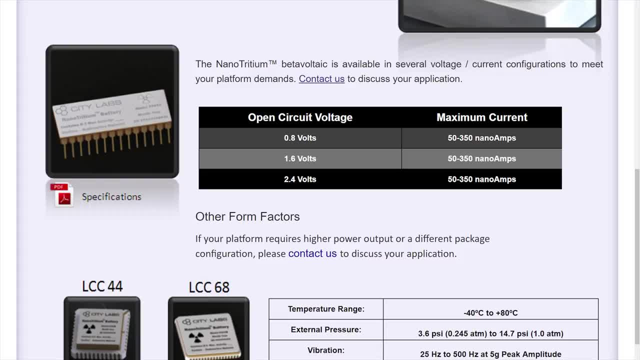 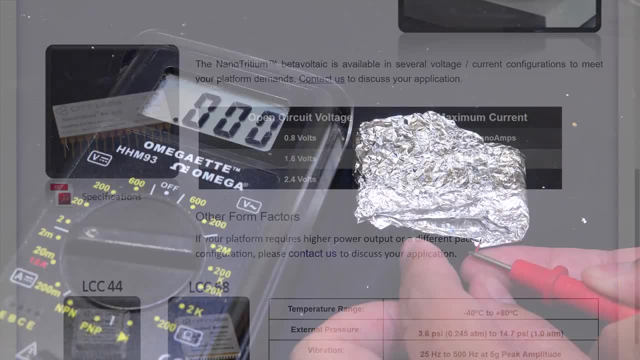 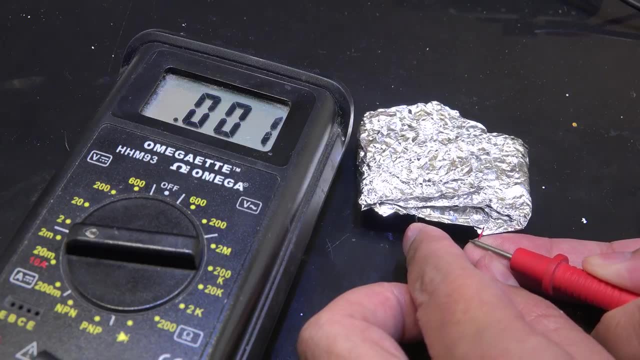 Or about 0.35 microamps, And it's about half the size of our device. We shouldn't expect to be able to beat actual nuclear scientists and engineers Now. i still want accurate performance numbers to compare to the professional device. We're going to need a way of measuring nanoamps of current at various voltages. 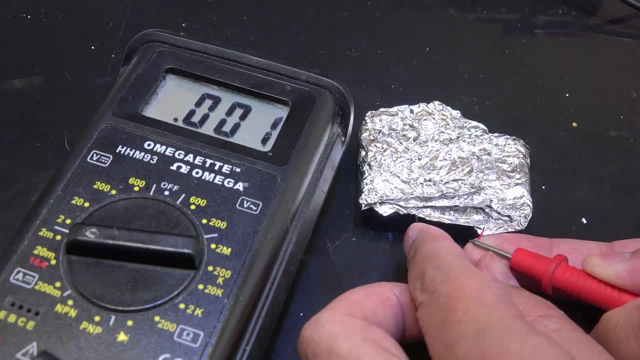 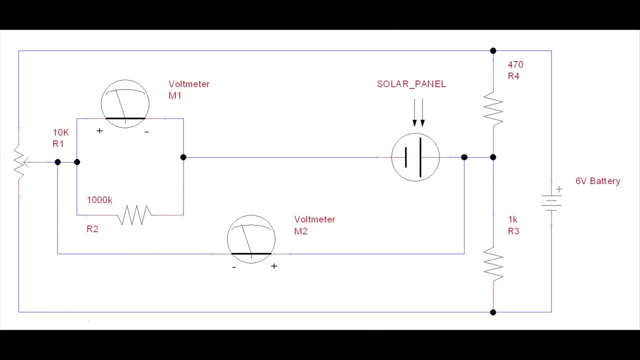 My meter can't go that low. I could buy a better multimeter, but i'll save some cash and build a circuit, And this is my circuit. Here is my circuit diagram showing how it works. It's more complicated than a simple ammeter circuit, because this circuit will also let us examine other performance characteristics, like the current versus voltage curve, and find the maximum value. 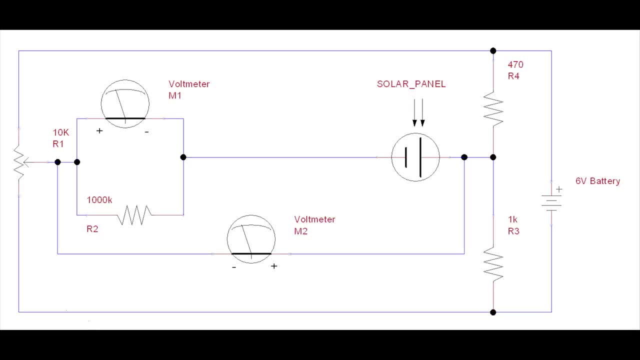 And this is my circuit. Here is my circuit diagram showing how it works. It's more complicated than a simple ammeter circuit, because this circuit will also let us examine other performance characteristics, like the current versus voltage curve, and find the maximum value. First, this potentiometer here, these resistors over here and this battery form a simple voltage source and divider that will allow us to impose the voltage on the nuclear battery. 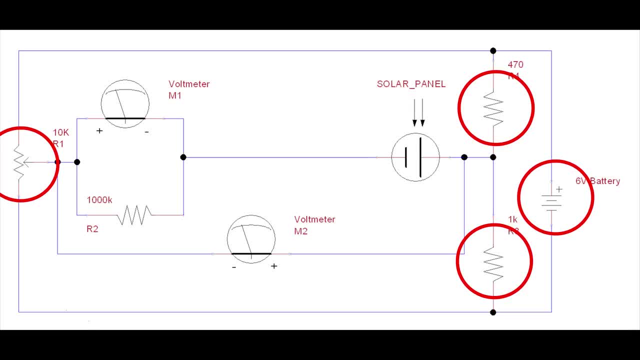 We'll be able to control the magnitude and even the direction of that voltage with this potentiometer. The voltage will be measured by this voltmeter i've inserted here Now to measure the current. we'll be using this voltmeter and this 1 mega ohm shunt resistor. 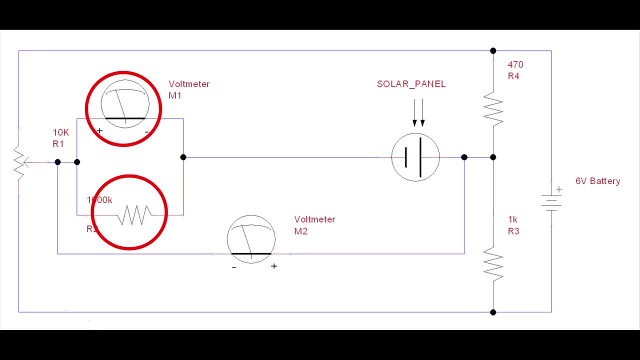 By using such a large resistor, the voltage difference across the circuit will be less than the current. The voltage difference across it, caused by nanoamps of current, reaches millivolt levels. A voltmeter can easily measure millivolt voltages, and thus we can calculate the current by simply dividing the observed shunt voltage by the shunt resistance. 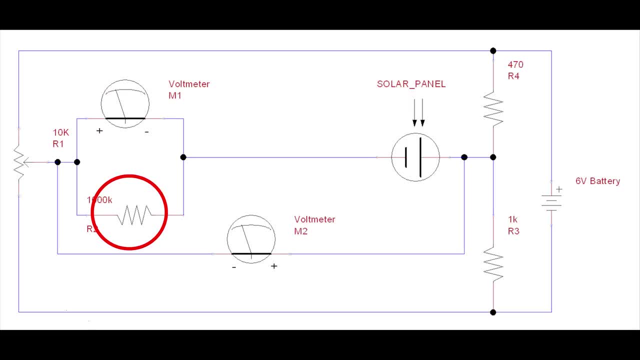 Now a special point i need to make. the shunt resistance is not just this 1 mega ohm resistor. There is actually a 10 mega ohm equivalent resistance across the voltmeter. Ideally, a voltmeter will have infinite resistance. 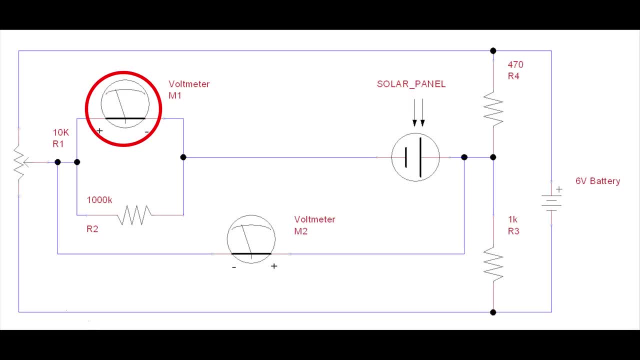 But practically a real voltmeter has some very high but finite resistance. So the actual shunt resistance is actually a combination of the voltmeter internal resistance and the external shunt resistance. Now we don't know exactly what the internal resistance is, but we don't have to. 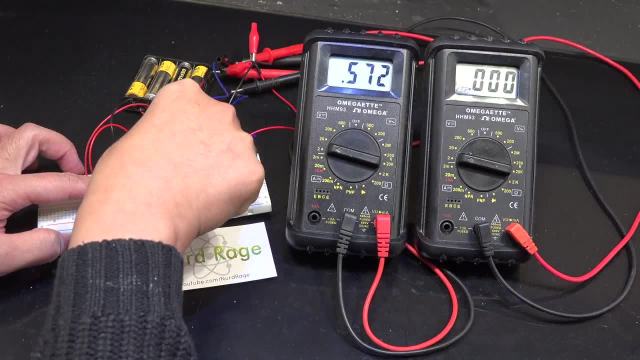 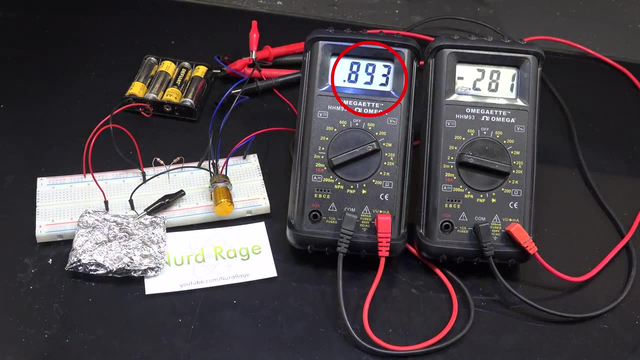 We can simply measure the combined resistance directly by connecting the other voltmeter to it, switching to ohm meter mode and measuring it on the mega ohm scale. That value there is the combined shunt resistance of the voltmeter and the external shunt and we can use that in our calculations. 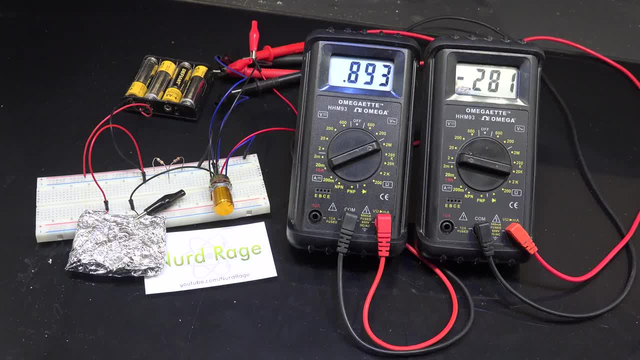 It's not often that the non-idealities of your multimeter will affect your circuits, but you need to be aware when they do. Now, at this point, you might ask if the voltmeter has significant error at the nanoamp current levels, wouldn't my measuring with this ohm meter also have errors in it as well? You're absolutely right. but in that case the makers of the multimeter know this and have calibrated the internal circuitry to compensate for that. So measurements, even in the mega ohm range, are still accurate to within 1 or 2%. Okay, now we know the total shunt resistance and record it in our lab notebook. 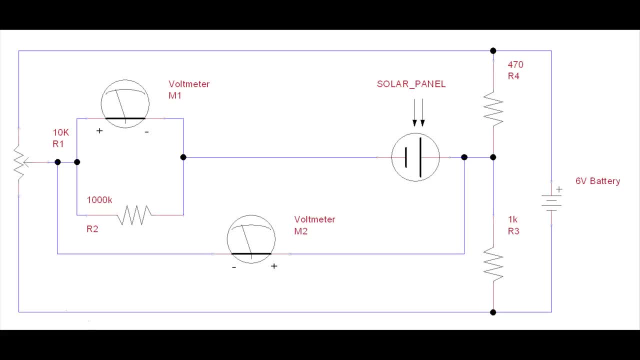 Let me reassemble my circuit Now. if you look at my circuit again, knowing how big the shunt resistance is, you'll notice something. I've put the voltage measuring voltmeter across both our current measuring shunt and our solar panel. If i want to measure just the solar panel, why am i putting it across both? 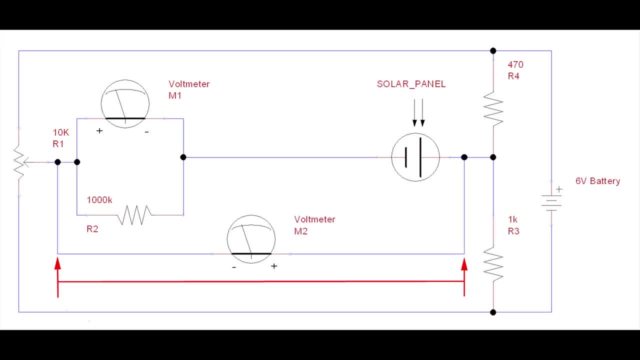 The voltage difference across them will be the shunt and the solar panel combined. Since the shunt voltage will be in the millivolt range, that would directly and significantly affect my results. So why am i doing that? Well, you can put the voltmeter directly across the solar panel. 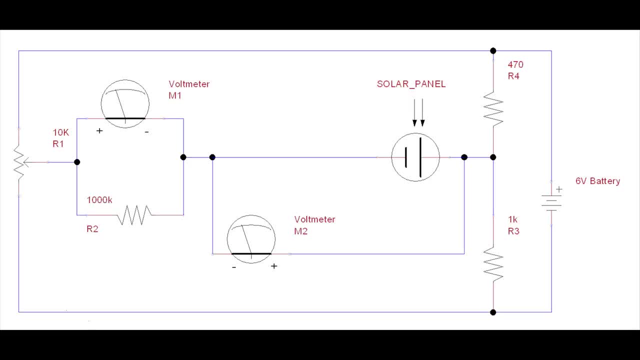 But this actually makes the measurement harder. Remember when i said the voltmeter itself has a large but finite resistance. Well, at nanoamp current levels, this affects the results of the voltmeter and the ammeter circuit. I can prove it here. 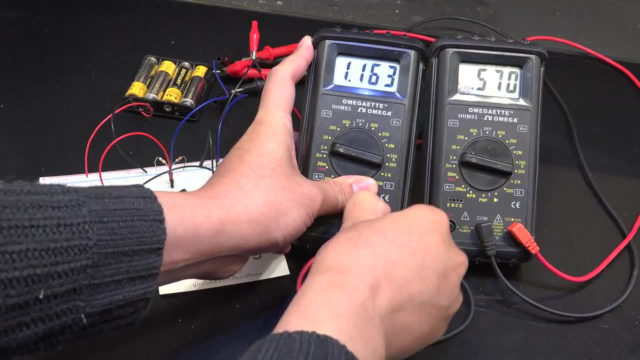 I've connected the voltmeter directly to the solar cell. As you can see, when i connect or disconnect the voltmeter, the ammeter shows a change. I've connected the voltmeter directly to the solar cell. As you can see, when i connect or disconnect the voltmeter, the ammeter shows a change. 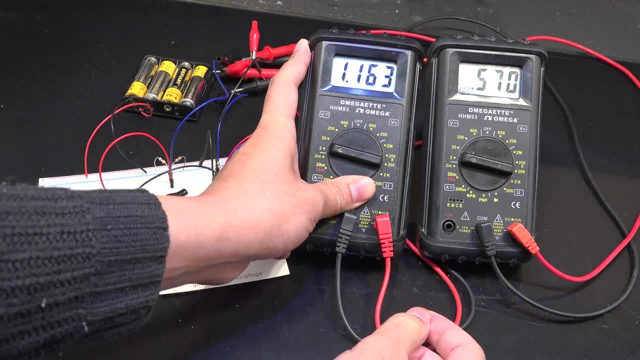 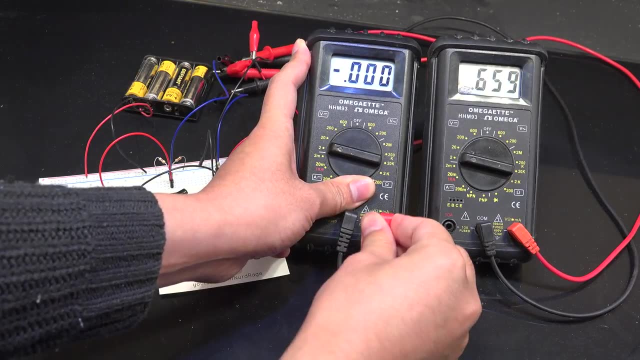 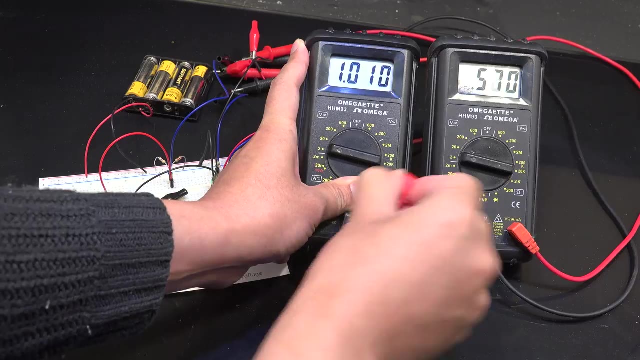 The current that is being drawn off by the voltmeter and its internal circuitry is significantly affecting the results. While it is possible to measure the internal resistance of the voltmeter and mathematically correct for it, it is mathematically simpler to measure the shunt voltage and the solar cell voltage together. 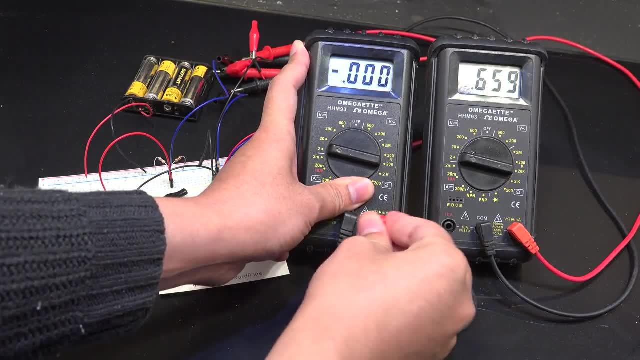 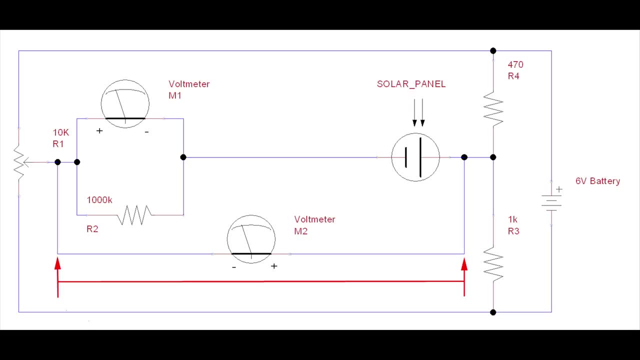 and just subtract the shunt voltage, which we can read off directly on the ammeter circuit. So why put the voltmeter on these points? In my case, though, since my current measuring at voltmeter is connected more or less backwards, I add the voltages rather than subtract, but the mathematical principle is the same. 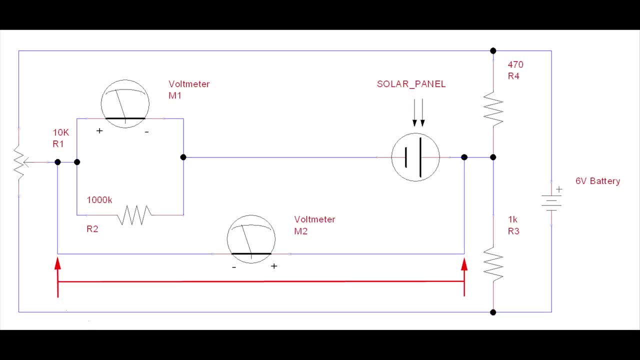 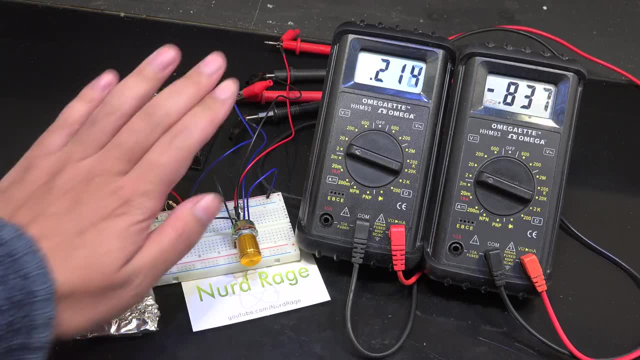 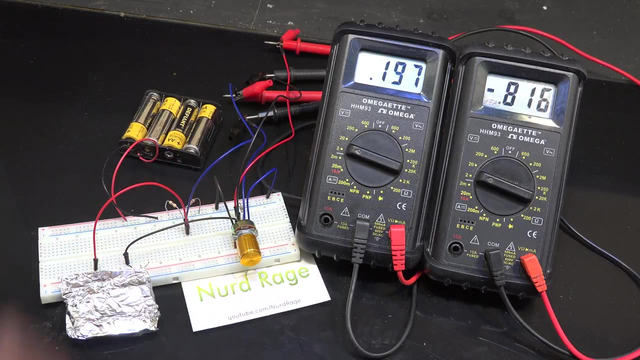 I put it in backwards so i can read the current on the positive axis. Now, before we start taking measurements, be absolutely certain no extra light is getting in, Just shade the aluminum envelope containing the nuclear battery to check. If the readings change then there is some light leaking in and you need to encase it better. 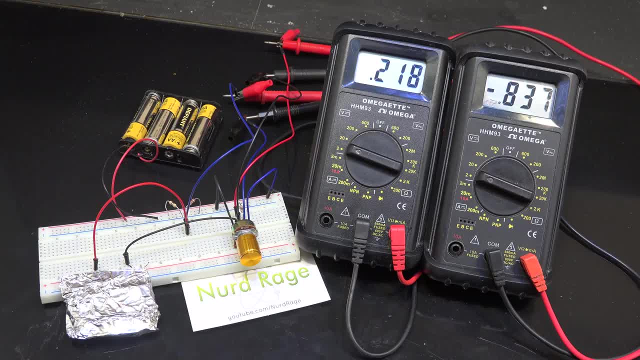 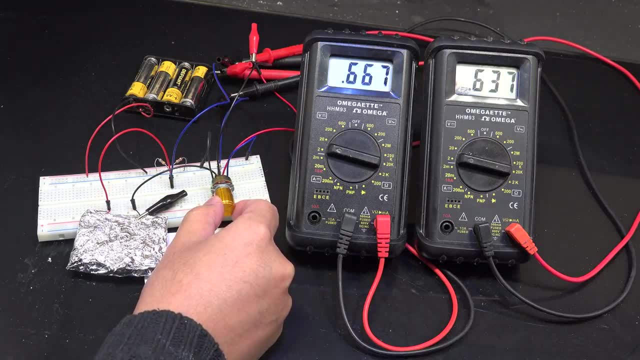 This was a problem in my earlier attempts, before i finally wrapped it properly. Anyway, we can start taking measurements. It's just a matter of reading off the voltages and rotating the potentiometer to the next voltage. We can sweep across the voltage range and get current readings on each voltage. 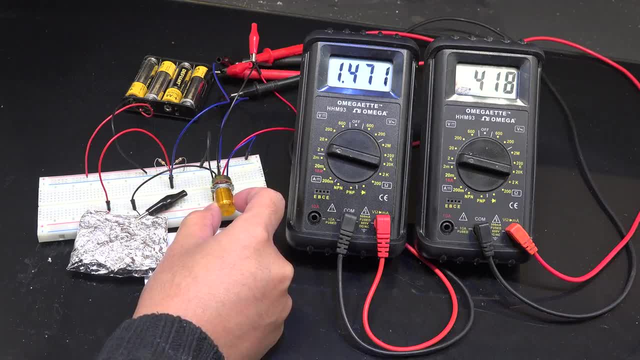 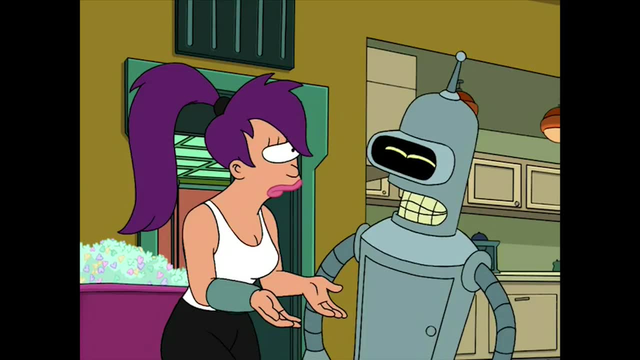 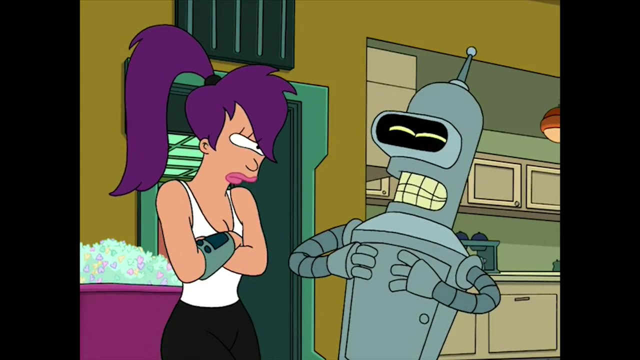 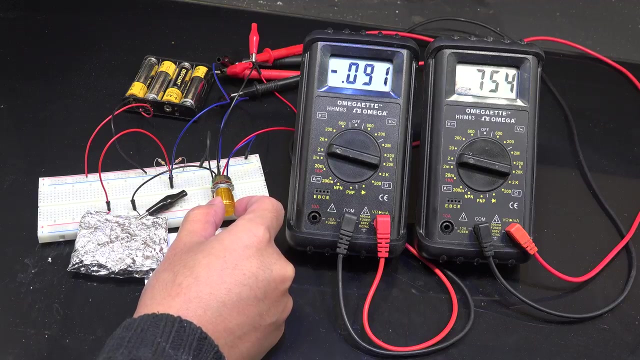 Granted, you have to sit down and take a bunch of data points, but it works. Now, at this point, i'm pretty sure you actual electrical engineers are reacting to my circuit like this. Oh wait, you serious. Let me laugh even harder. Yes, i know a completely automated circuit would have some sort of digital voltage regulator and a couple of ADC's and could sweep all the voltages in a few seconds and record them in a computer. 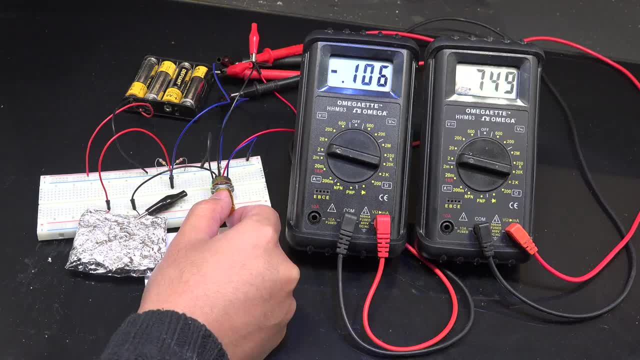 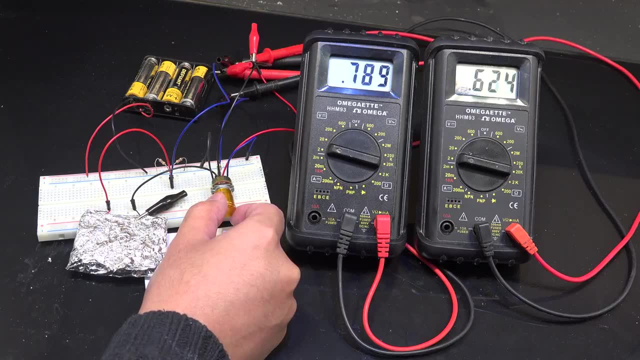 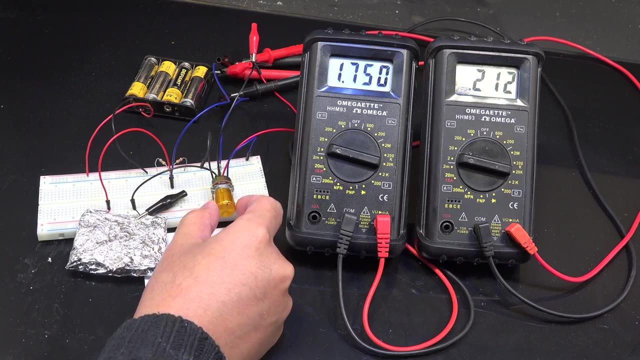 I'm sure there are arduino or raspberry pi devices and shields that handle everything in one go, But then again, that's why i'm the chemist and you guys are the engineers. You may continue laughing. Okay, once we collect all our data, we can now start processing it. 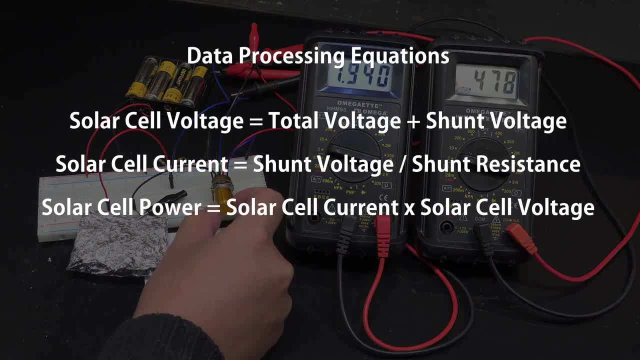 We add together the shunt voltage and the total voltage to find the solar cell voltage. I must emphasize again: i can add them because i wired the current measuring voltmeter in the opposite direction of the total voltage measuring voltmeter. If it were in the same direction you'd subtract the voltages. 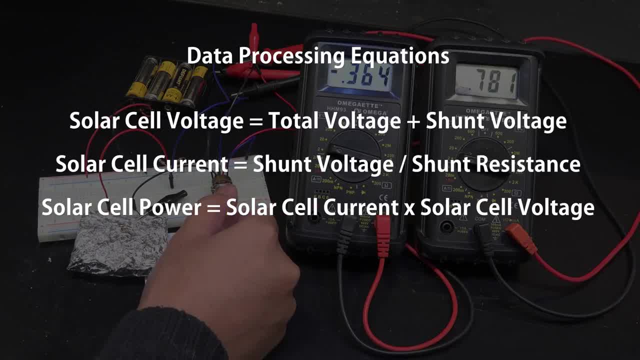 Now to find the current, we divide the shunt voltage by the total shunt resistance. that we found to be around 0.89 megaohms for the combined external and internal resistors. Finally, we find the power by multiplying the total voltage and the total voltage. 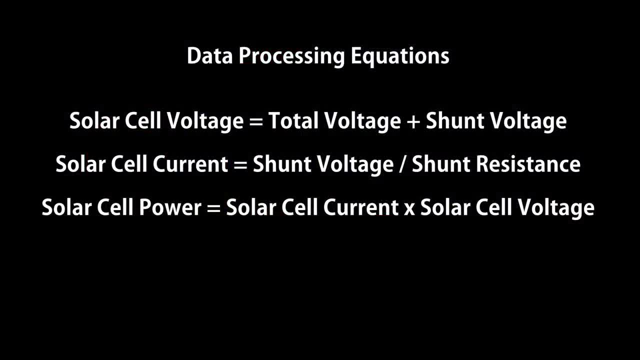 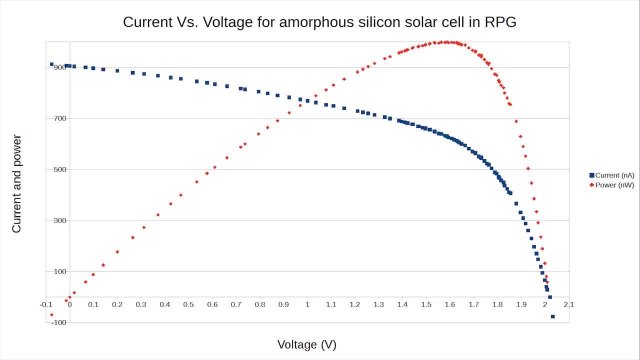 Then we multiply the solar panel voltage by the current. Now we plot the current and power versus voltage, And that is beautiful. There is nothing quite like plotting scattered data points and watching the underlying science emerge through the curves. One of the tiny little joys of research. 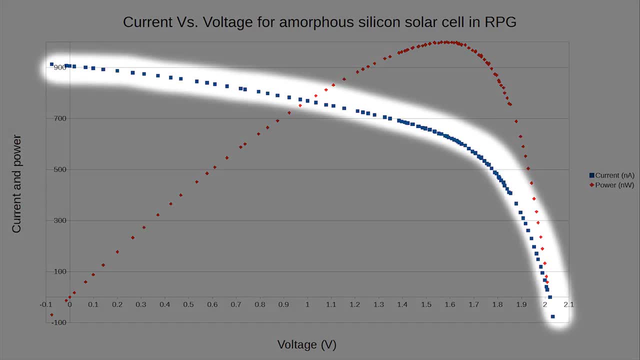 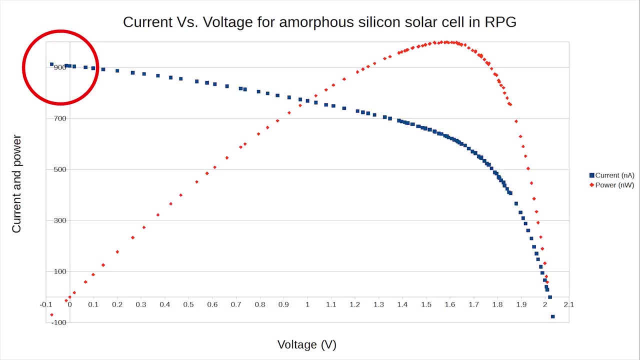 So let me explain what we're seeing. This blue line here is the current versus voltage. The current at zero volts represents the short circuit current and is the maximum current the solar cell can produce. Now to the right here, where the current is zero, is the open circuit voltage. 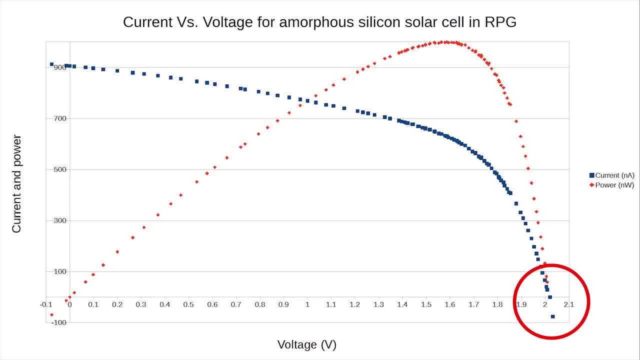 This is the voltage if the solar cell is completely unloaded. As you can see, we can draw more and more current very easily until we reach a kink or a knee where the solar cell can no longer generate much more current to meet demand. At that point the voltage decreases rapidly, with only modest increases in current draw. 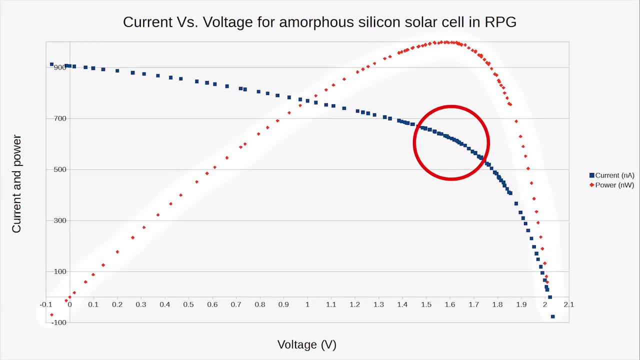 This is the maximum power point and can be found easily by simply plotting the power output versus voltage. We can see it here. We can see it as this orange plot. The very top of the curve is the maximum power point and, as the name suggests, you get the most power from your solar cell if you design your circuitry to load your solar cell to this voltage. 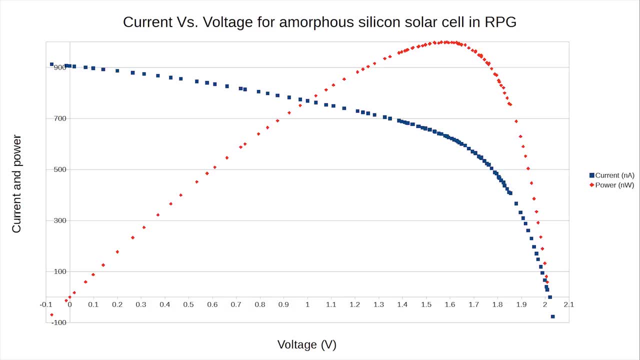 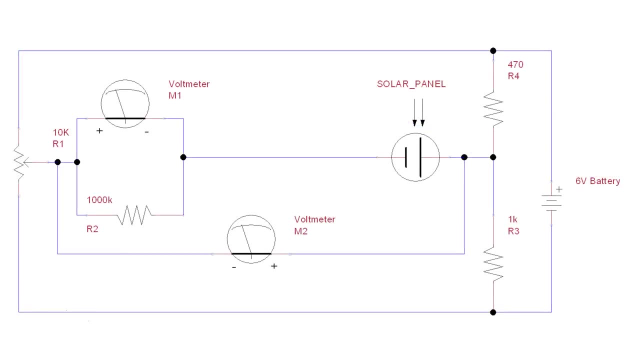 In this case around 1.6 volts. Now you might be wondering how i can have numbers into the negative region of my chart. My measuring circuit can apply voltages beyond the limits of the solar cell. There is nothing particularly special about those limits, so the trends in solar cell behavior continue. 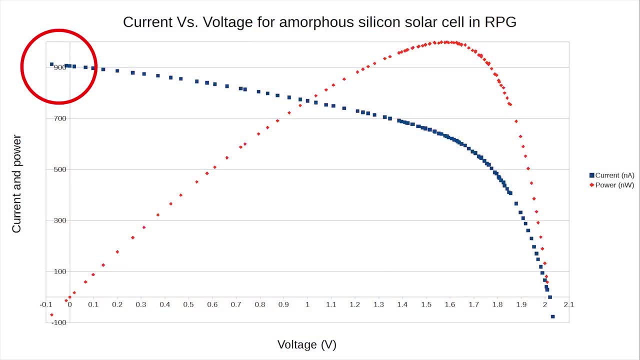 We're just now draining the voltage. The voltage is really going to be all over the board. The voltage is going to be with the current coming in rather than the current entering, so we're draining power rather than generating it. At the negative voltage region we have a very sensitive light detector. 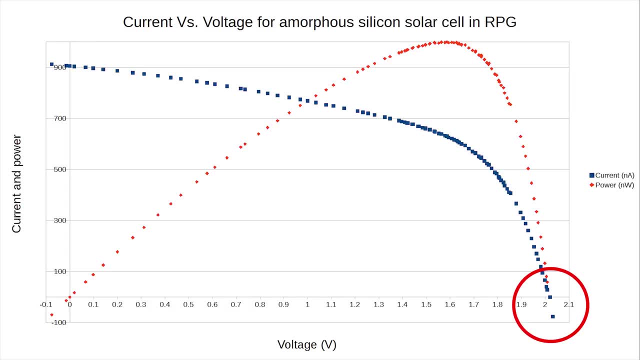 And this is the basis of some photodiode detector circuits. Beyond the voltage maximum is where the light emitting diodes work and instead generate light rather than absorb it. For a solar cell, however, it won't actually emit light, since it's not designed that way, and it will just heat up. 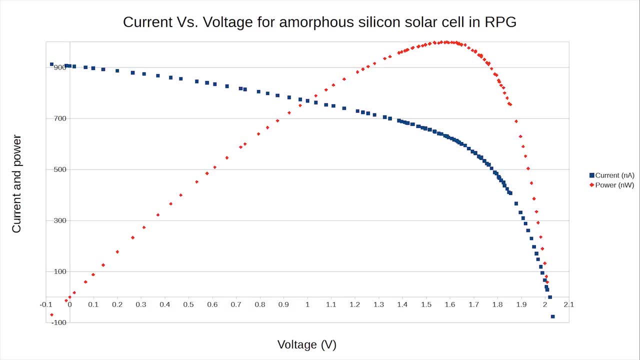 Anyway, on the whole, i'm very satisfied with these results. We were able to measure the performance characteristics like short circuit currents and maximum per second. We're getting almost exactly 1 microwatt of power. Let's see if we can do better. 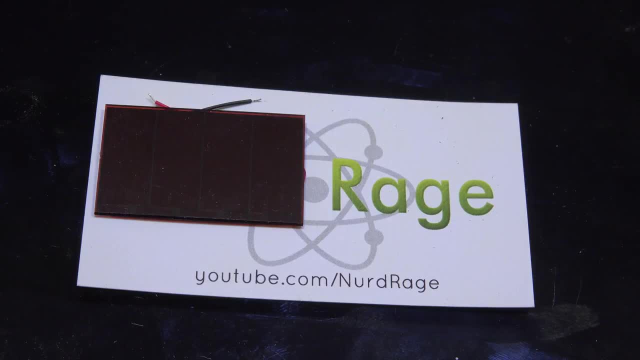 Now, amorphous solar cells are not very efficient- about several percent, and that's about it. If you've looked into solar cells, you know there are monocrystalline solar cells that you can buy at around 20% efficiency or higher. 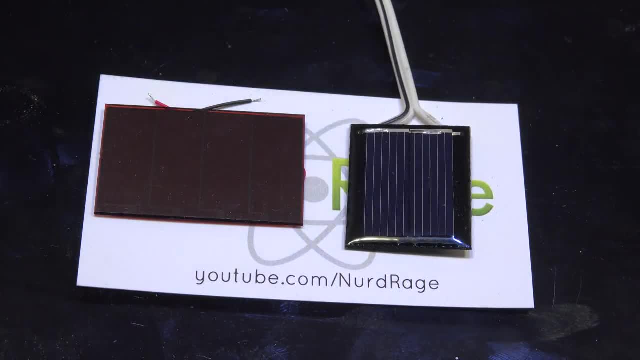 So let's try that and see if we can do better. Now i know what you're thinking. this monocrystalline solar panel i'm using is much smaller than my amorphous cell. It won't be a fair comparison because it will generate less power than a solar cell of equivalent size. 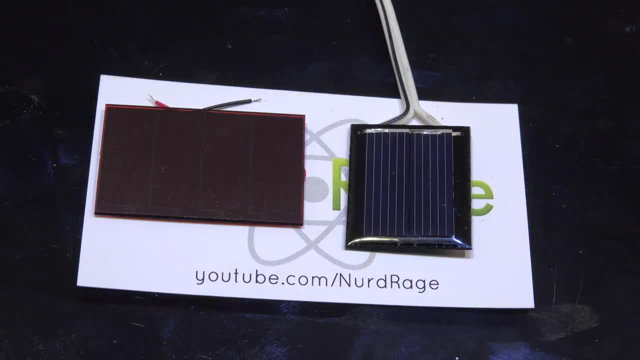 You're absolutely right, but we can scale our results by measuring for area. I measured the monocrystalline panel to be 450mm2 in size And i measured the amorphous panel to be 1092mm2 in size. 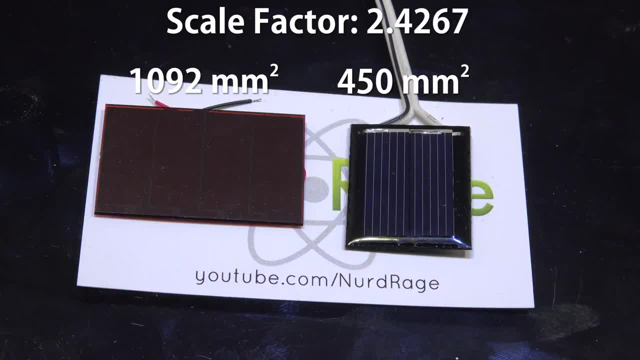 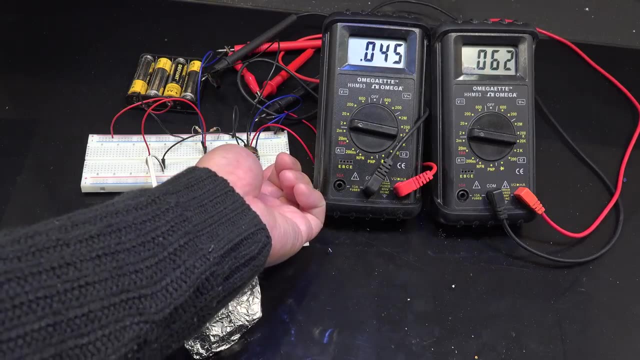 So the scaling factor is around 2.4267.. I just need to multiply the current by that number and they'll be comparable. Voltage is constant regardless of surface area, so it doesn't need to be scaled. So i've assembled the monocrystalline solar panel into our measuring circuit. 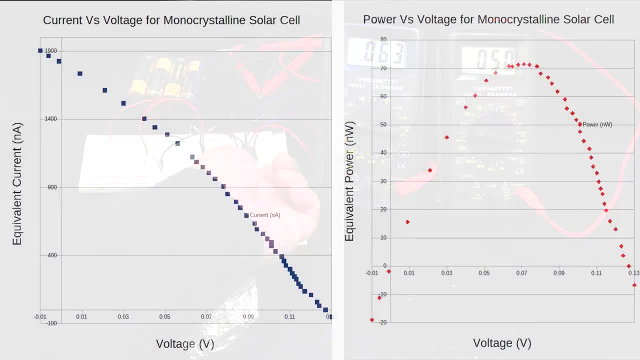 Let me gather the data and start plotting, And here are our results. As said before, i'm multiplying the current by the scale factor so we can compare them to our amorphous silicon panel. I had to put the power and current in separate charts, since the numbers were so different. 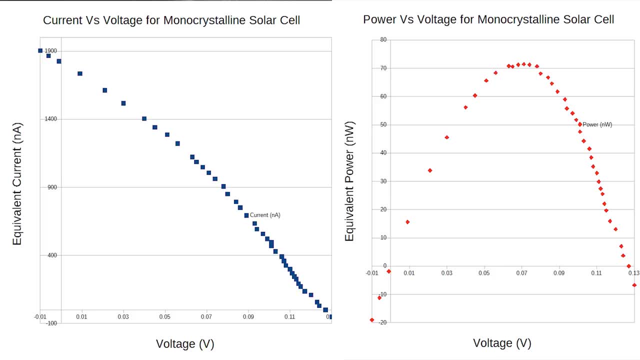 Now, the monocrystalline panel produced a lot more current compared to the amorphous panel, But the voltage max was much less. We can attribute some of this to the monocrystalline panel having fewer individual solar cells inside of it. 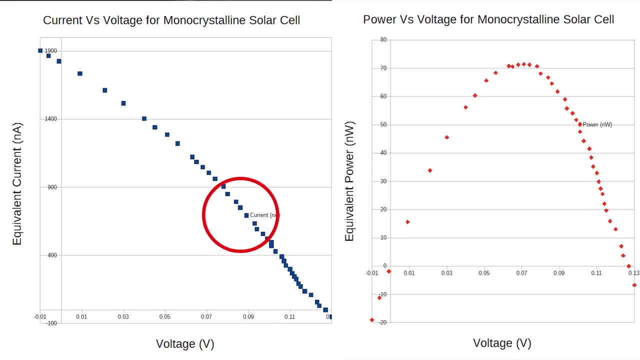 But the most interesting difference is this fairly constant slope, for the current trace and maximum power point is much lower. At best we're only extracting 71 nanowatts, And that's already been scaled to match the size of the amorphous panel. 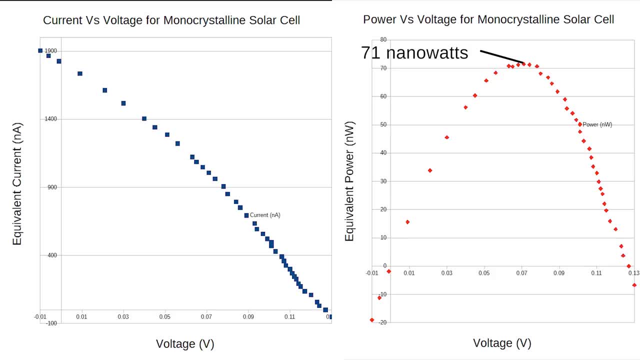 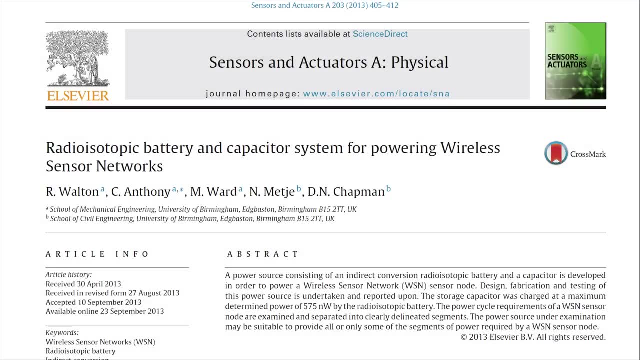 This monocrystalline panel is only giving us 7% of the performance. At first i thought i was doing something wrong, But i looked up the research by other groups and found this is a fairly well known observation. High efficiency monocrystalline solar cells are only efficient in very bright light. 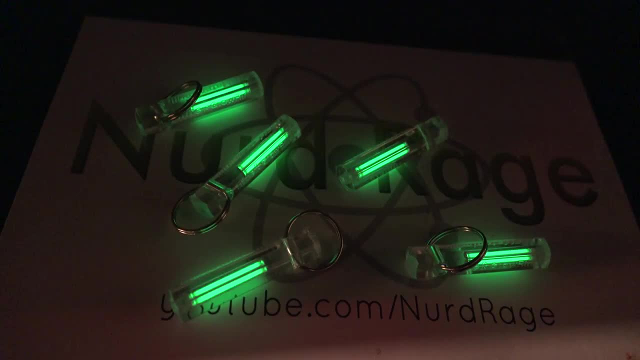 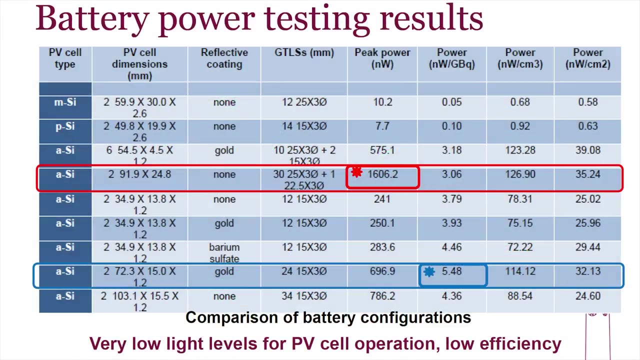 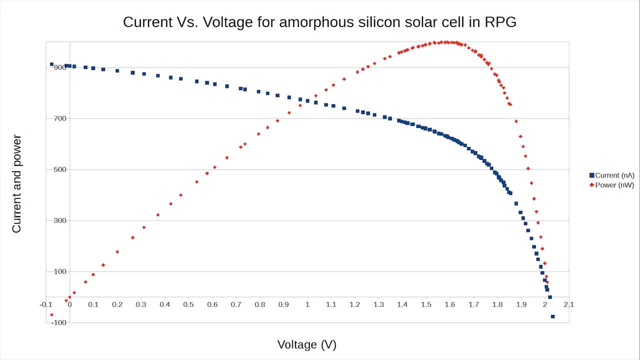 In very dim light, like the weak glow of these tritium vials, they actually perform very badly. Amorphous silicon solar cells, while being very inefficient in bright light, give much better performance in low light conditions. In thinking about this, i've actually seen this before, but never really noticed it. 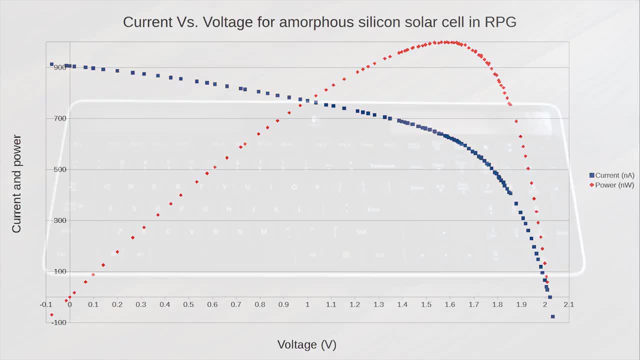 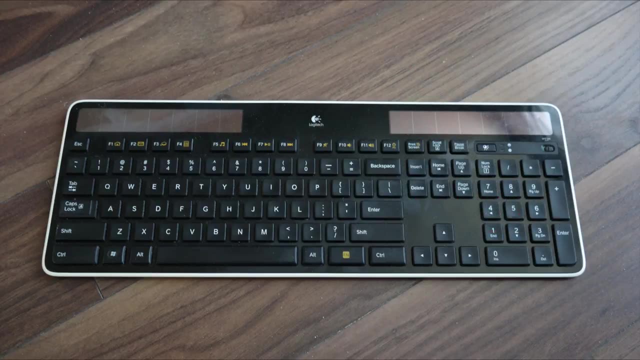 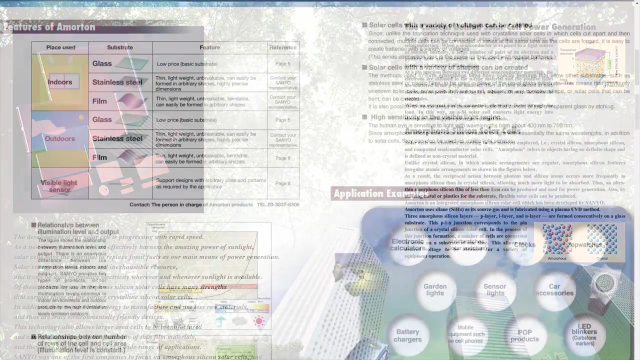 Devices meant to work indoors with low light, like the solar keyboard or calculators, almost exclusively use amorphous solar cells. I've never seen one use monocrystalline solar cells. I even found this advertisement page extolling the virtues of using amorphous solar cells for low power. 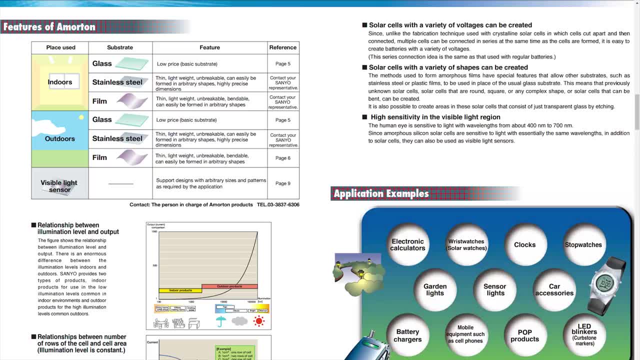 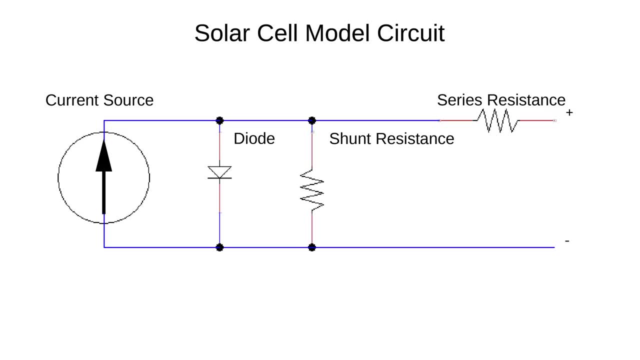 So apparently everyone knew that amorphous solar cells are better for indoor light, except me. Now, to understand why this is, we can look at this solar cell model study. A solar cell behaves like a current source in parallel with a diode and shunt resistor. 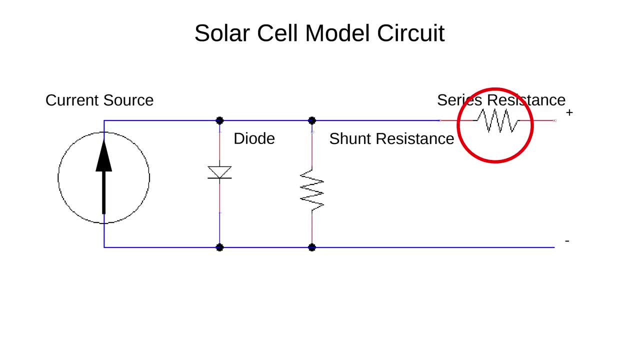 There is also an equivalent series resistance, but for this analysis we can ignore this. Now, the shunt resistance isn't an actual device you can find. It's just a representation of all the combined properties of the solar cell, like the crystal structure defects, purity of the silicon and so on. 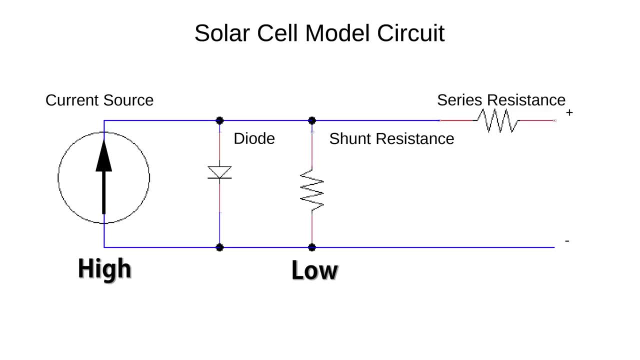 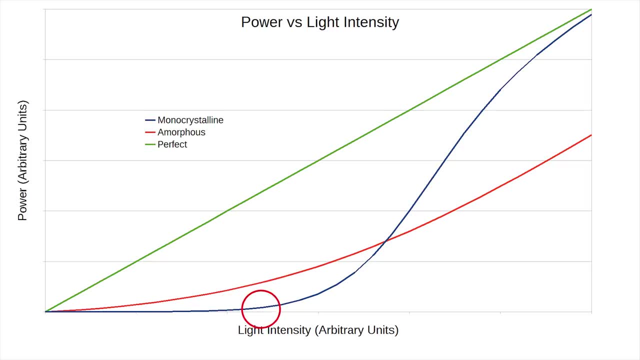 In a monocrystalline solar cell, the current source is very powerful and produces a lot of current, but the shunt resistance is rather weak. So at small power levels, like low light, it dominates the circuit and shorts out what meager power is available. 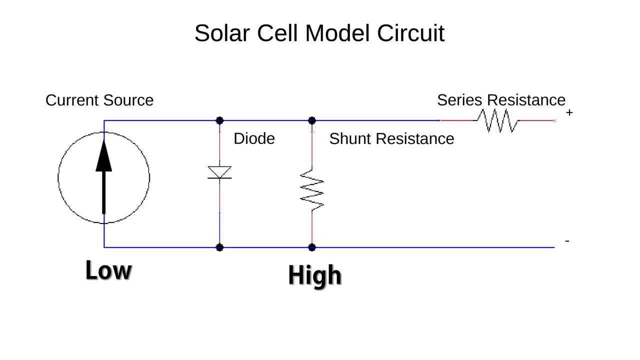 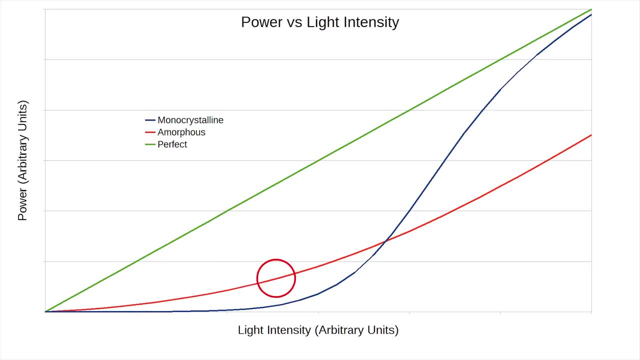 In an amorphous solar cell. the current source is weak but the shunt resistance is huge so it has very little effect at low light. So for low light conditions the amorphous solar cell produces more usable power than the monocrystalline one. 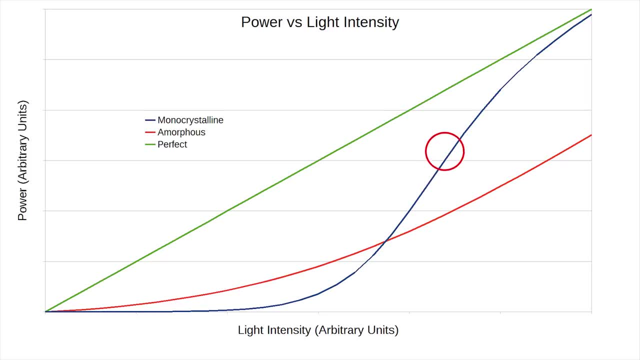 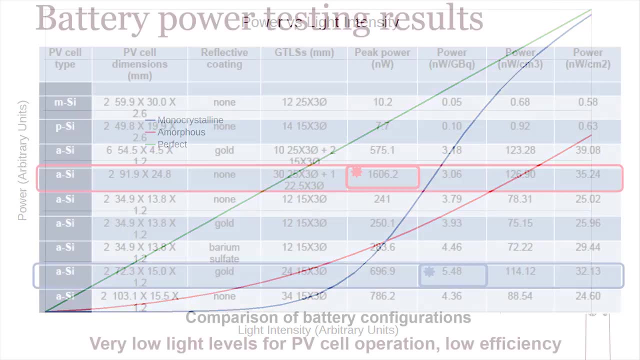 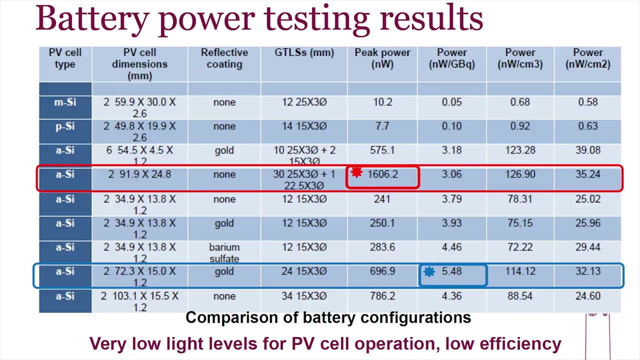 For bright sunlight, though the massively powerful current source dominates the circuit in a monocrystalline solar cell, And thus they are used in bright sunlight Where they give the most benefit. Anyway, I was going to try other solar cell types like polycrystalline, but it seems the consensus among all the other researchers is that amorphous solar panels are the best for low light nuclear batteries. 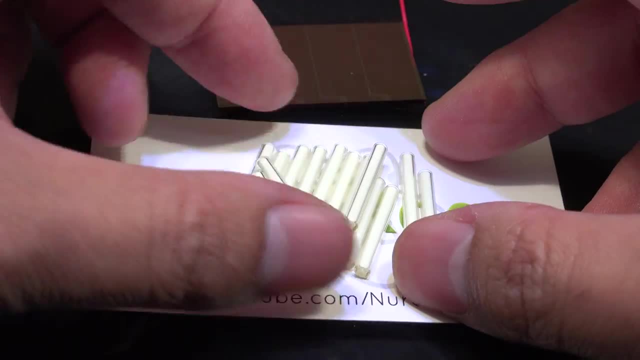 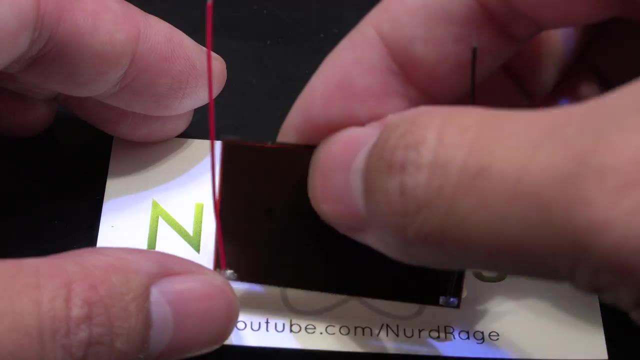 So i won't bother. Okay, since we're going to use amorphous solar cells exclusively, let me rebuild it. You might be wondering if different colors or shades would be better. I was only able to get discounted tritium vials for the color green, so that was all i was able to test. 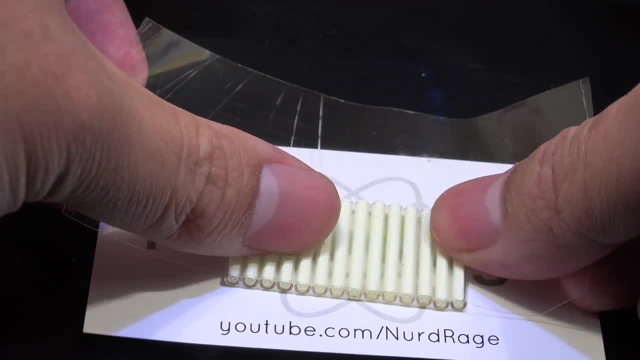 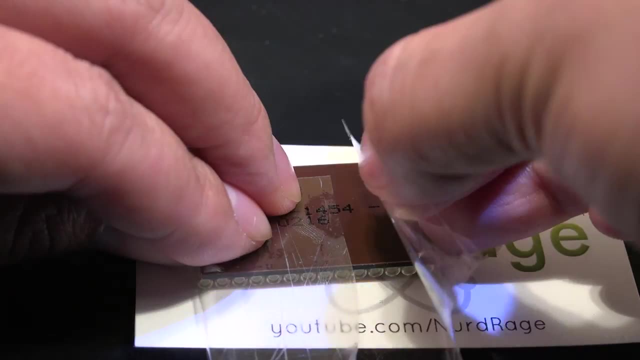 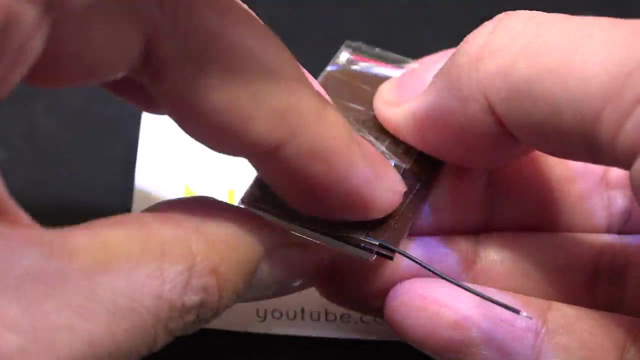 The articles i read from other researchers mostly used green and some tested blue, but i didn't find any broad, rigorous testing to determine the relative qualities of all available colors. So that's something you could try looking into if you want. As for shapes, i've seen rectangular tritium lights, but those seem to be more expensive for the same given area. 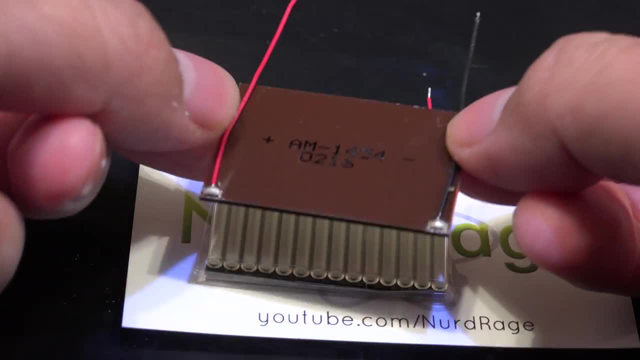 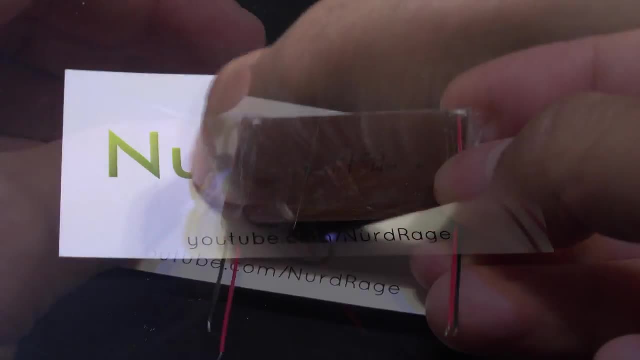 Now we should be able to almost double our power output. doing the obvious, sandwiching a second solar panel on the device, And there we go- a double sided nuclear battery. Once again, i'm going to put the unit in foil to protect it from external light, so we can get accurate measurements. 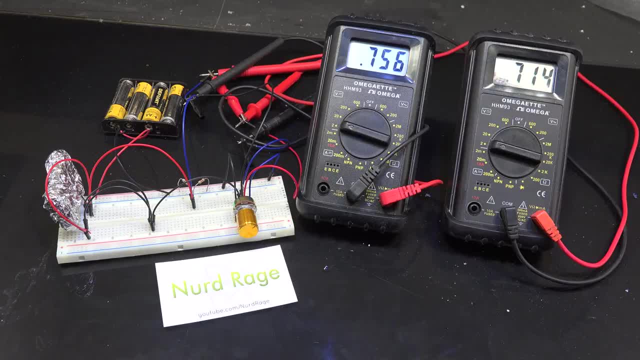 I've inserted the device back into my measuring circuit. Now i've connected the solar cells in parallel to get increased current. You can connect them in series for increased voltage if you want. The total power will still be the same, Running the voltage sweep again. we then plot the data and see how we did. 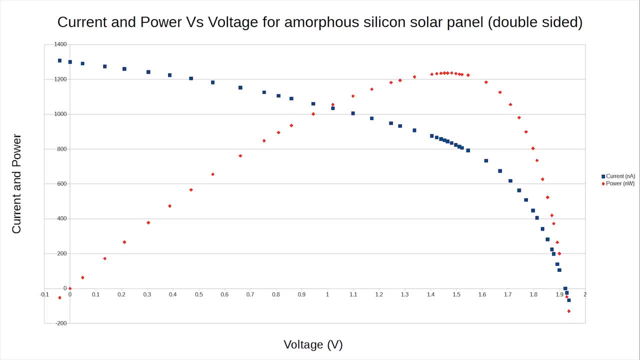 Interestingly enough, rather than getting twice the maximum power, we're only getting around 23% more. The maximum power is about the same. The power output is 1.23 microwatts rather than the 1 microwatt of the single panel device. 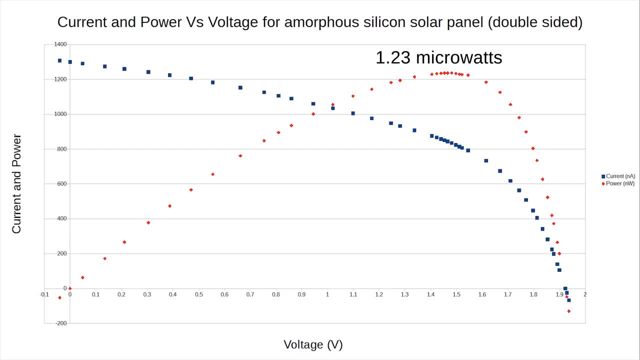 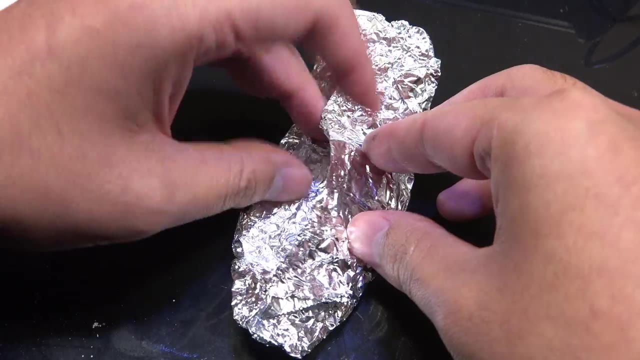 At first i thought i did something horribly wrong and rechecked my connections and work Turns out this data is correct. The reason why the single panel nuclear battery attempt had such a good power rating was because the aluminum foil i used to block the light actually reflected the other side of the tritium vials and returned the light back to the solar panel. 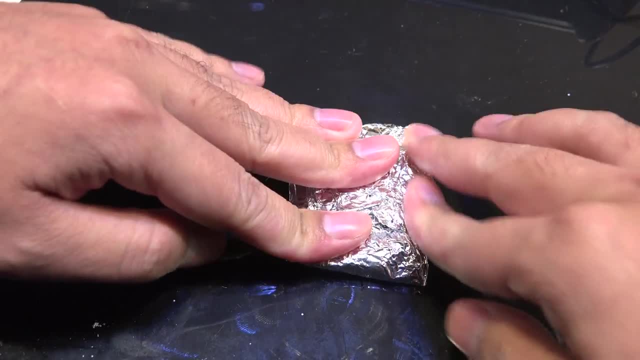 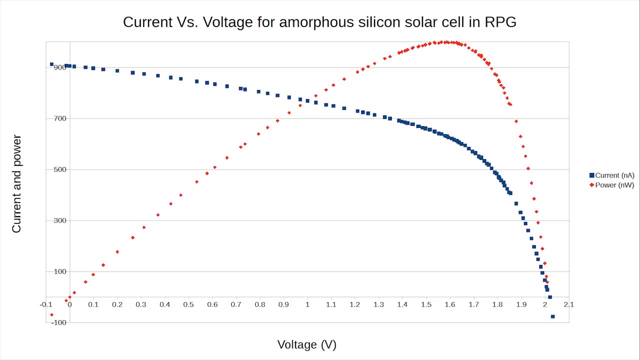 Now it had to go through the tritium tubes again, so it lost some power and thus didn't work. The double panel device didn't give the same power as a double panel device, but it still gave more than half a double panel device. 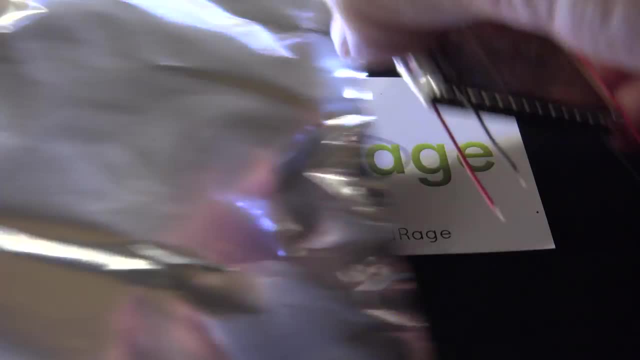 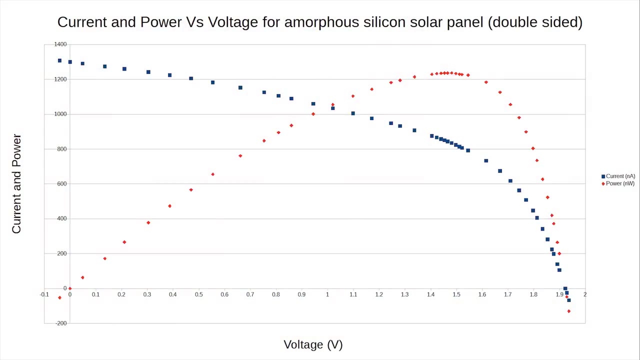 A good 60% more power. In my double panel device there is no reflection, so we're not getting that boost and thus not getting double power. Still, a greater than 20% increase is not negligible and worth keeping the extra panel, since that's still cheaper than 20% more tritium vials. 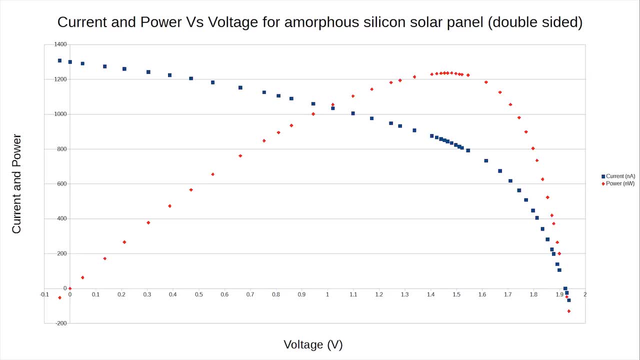 Now that we have our relatively optimized device, let's compare it to the professional one. Now. beta-voltaic technology is different from photovoltaic technology, but it should have a maximum power point as well. Unfortunately, city labs don't give us a current voltage graph like mine, so we don't know what the maximum power point is. 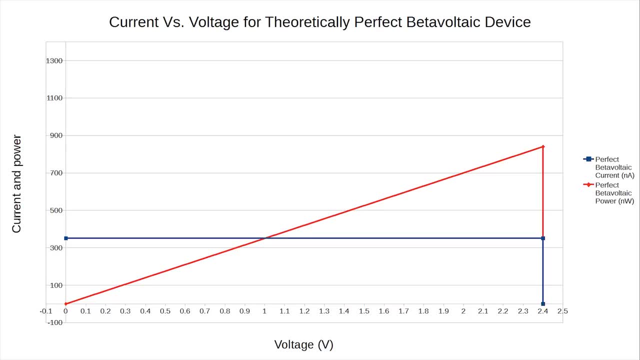 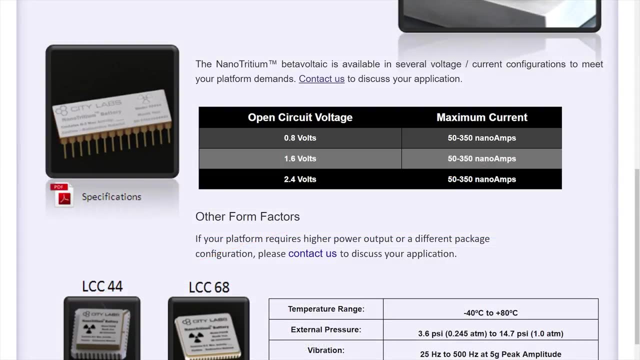 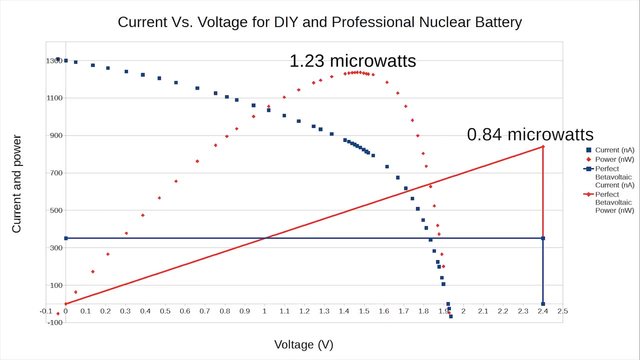 But let's give them the benefit of the doubt and assume they have perfect technology And their device gives perfect power. According to their specifications, they can provide 350 nanoamps at 2.4 volts or 0.84 microwatts. Our device at 1.23 microwatts is actually better than the professional device. 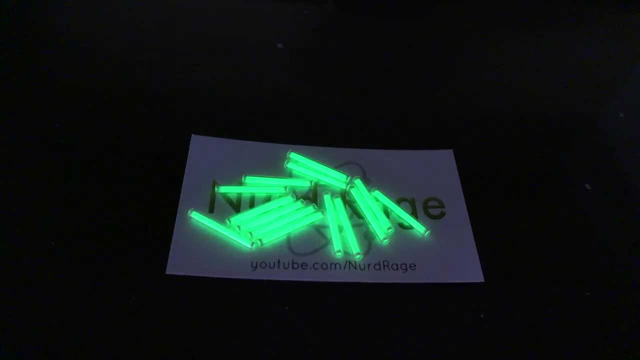 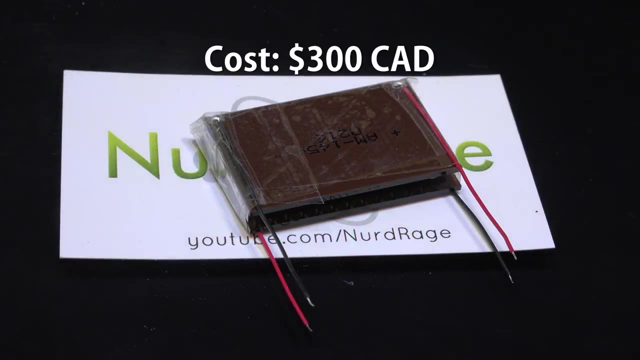 And we haven't even factored the cost yet, While i got my tritium vials for a steep discount. if you bought the components and the tritium vials at market price, then cost comes out to about 300 canadian. 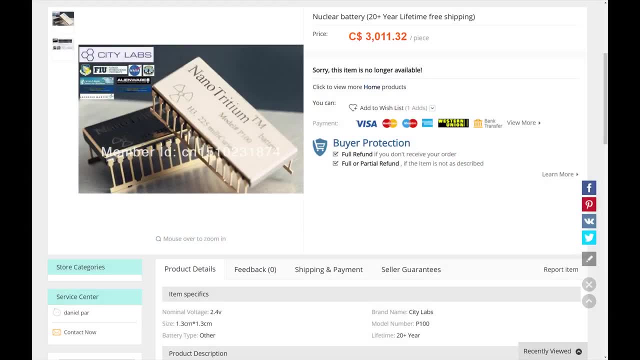 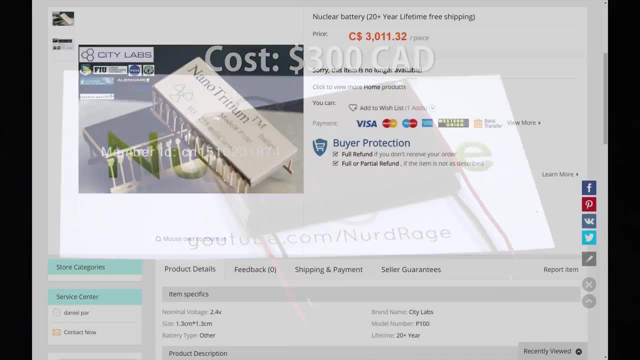 Meanwhile, the reseller was selling the city labs device for 3000 canadian. For that price we could build 10 of our devices. That being said, the city labs device is a bit expensive. The city labs device does beat mine in terms of size and weight. 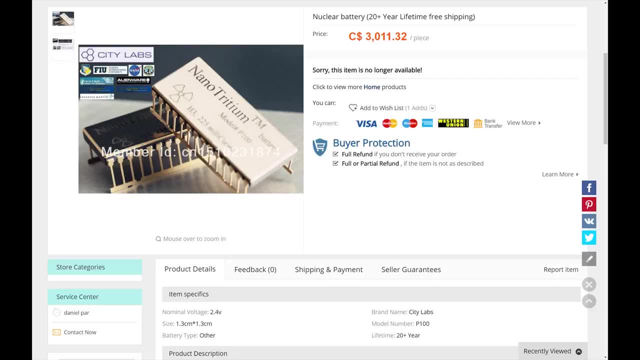 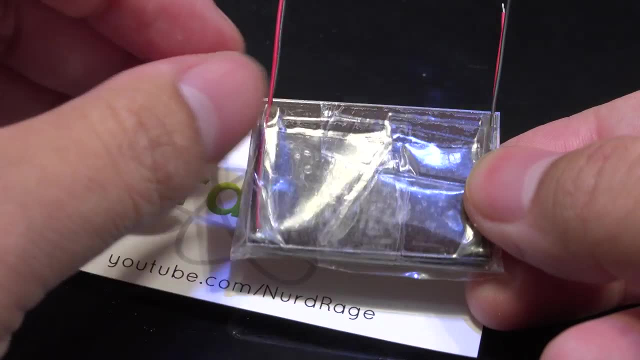 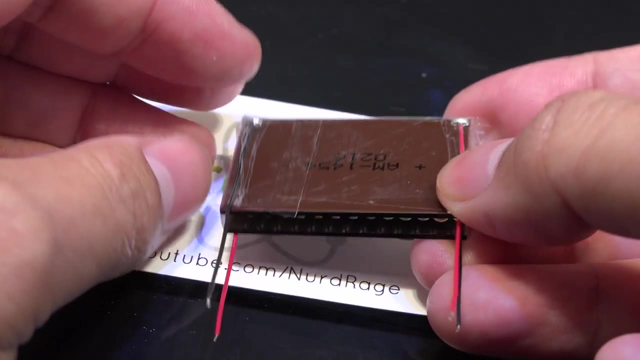 It is both smaller and lighter, and that could be an important consideration in devices where that is a premium, like spacecraft, or in medical devices like pacemakers. Nonetheless, i'm totally blown away. I'm not even an electrical engineer, let alone a nuclear engineer, and i've got something that is both cheaper and more powerful than the professional version. Now why is their stuff more expensive? They got two things working against them. First, they need nuclear regulatory approval. They need to be able to build and sell their devices. I'd imagine getting the legal paperwork done and meeting nuclear safety standards is not exactly cheap. 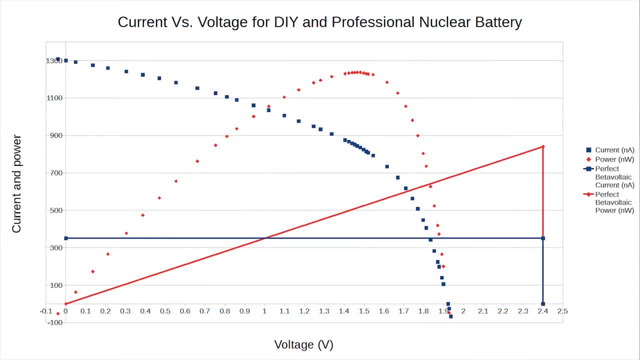 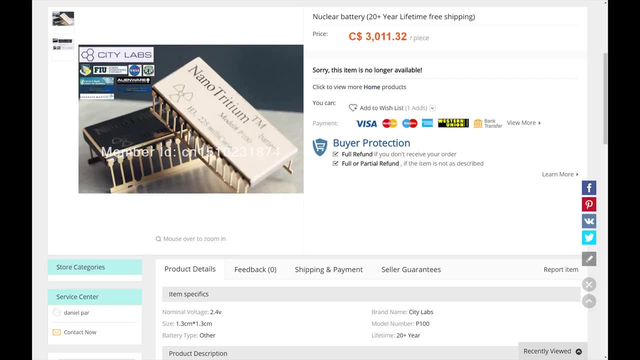 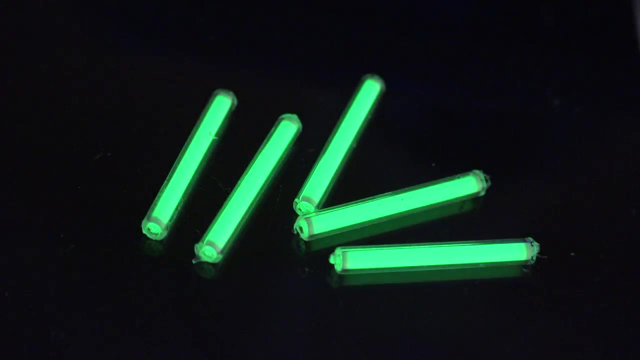 Second at just 0.84 microwatts. the number of applications isn't that high. It's unlikely they're selling in massive volumes, So they need to charge more per device to stay in business. We kind of cheat in that tritium vials are mass produced in large quantities for all sorts of uses, so economies of scale and the free market have made them affordable and well within the reach of the average person. 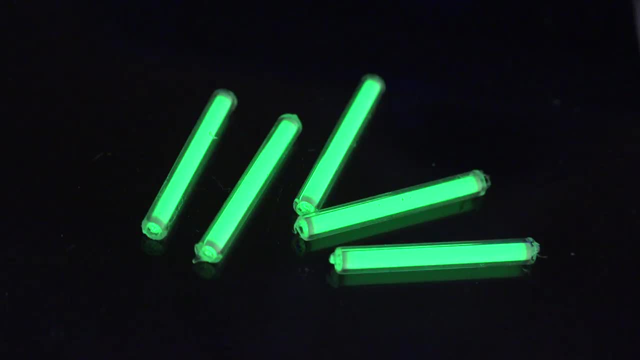 We kind of cheat in that tritium vials are mass produced in large quantities for all sorts of uses, so economies of scale and the free market have made them affordable and well within the reach of the average person. We kind of cheat in that tritium vials are mass produced in large quantities for all sorts of uses, so economies of scale and the free market have made them affordable and well within the reach of the average person. We also don't need nuclear regulatory approval to get them. Anyway, at this point you're probably wondering: how long does this last? Well, tritium has a half-life of 12.3 years, So ideally this should gradually have its power output every 12.3 years. 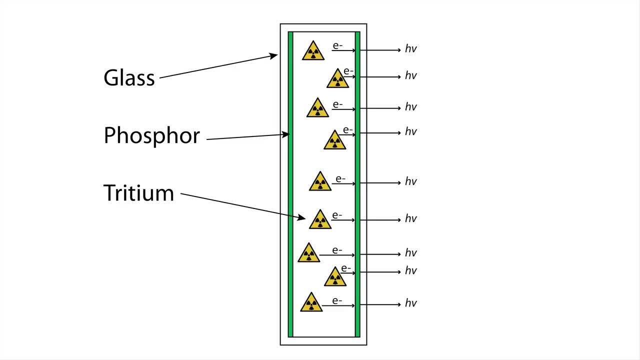 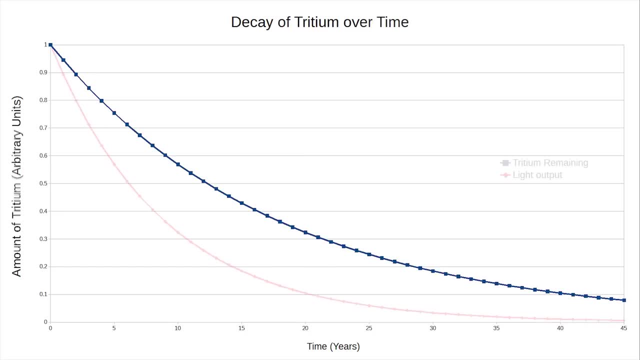 But there is another decay mode. the phosphor in the tubes themselves are constantly being bombarded with beta radiation and they will decay as well. So the total power output will decay faster than what the tritium half-life suggests. I don't know what the rate is, but it's something to keep in mind if you want to use this device for the very long term. 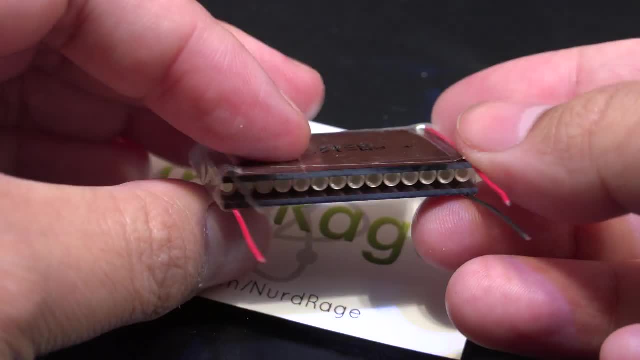 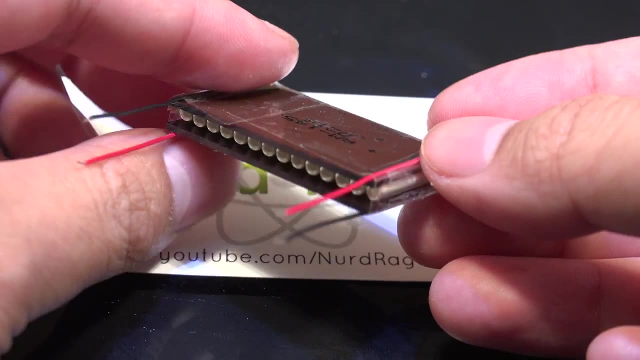 I also recommend using a better case than plastic tape. A custom metal box is best for the long term. So what can we power with this? As i said before, this is meant for extremely low power devices, where longevity and reliability are absolutely paramount. 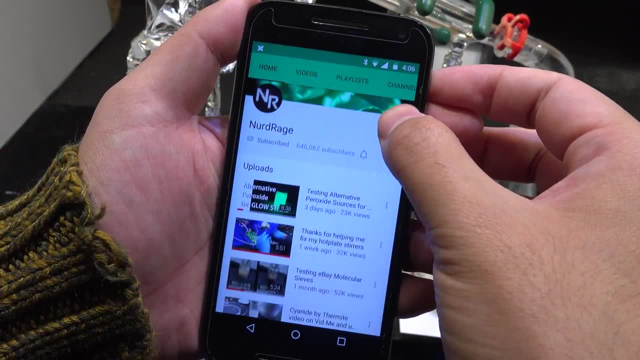 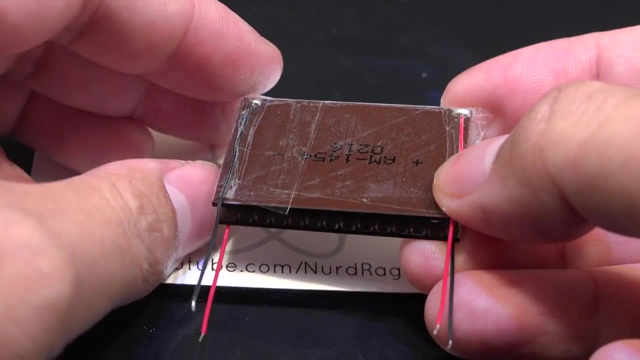 For comparison, if we want half a watt, which is enough to run a low end cell phone, we'd need 400,000 of these, Or about 120 million Canadian dollars worth. If your expectations weren't crushed already, they should be now. 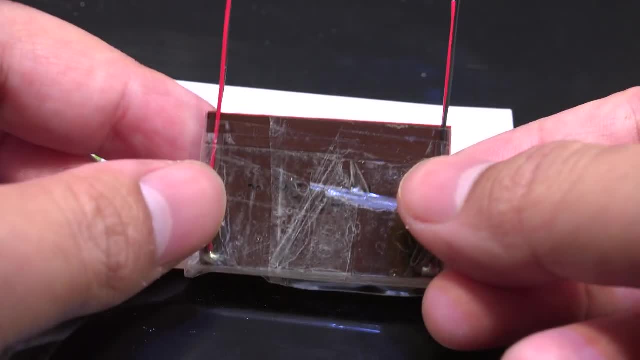 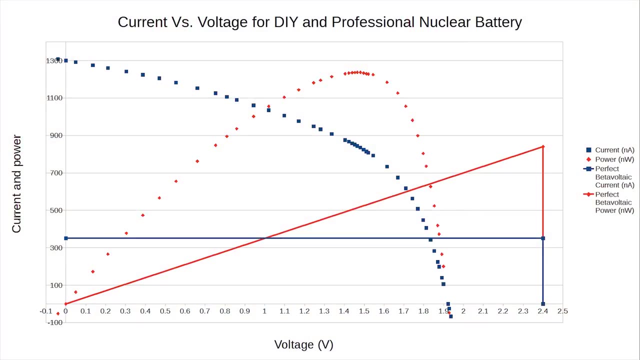 Now, i did want to use these for something, but i'm not an electrical engineer, so i can't build the nanowatt level circuits that would take advantage of this battery. But i'm sure all you guys have better ideas and we should discuss them in the comments.